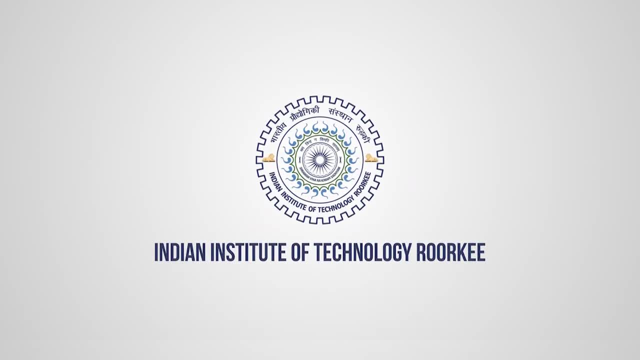 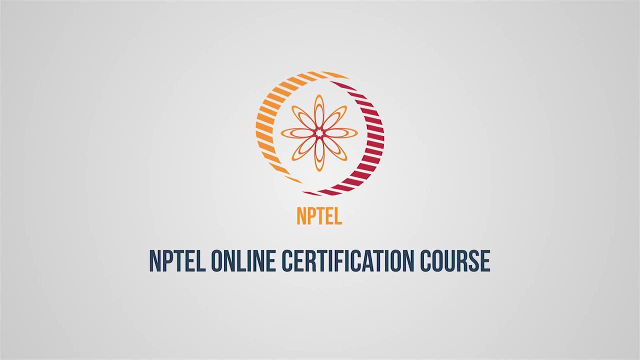 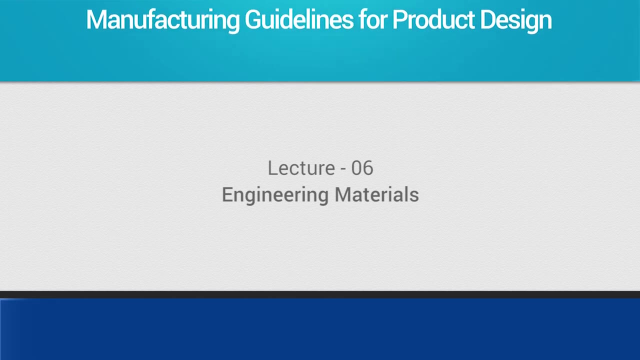 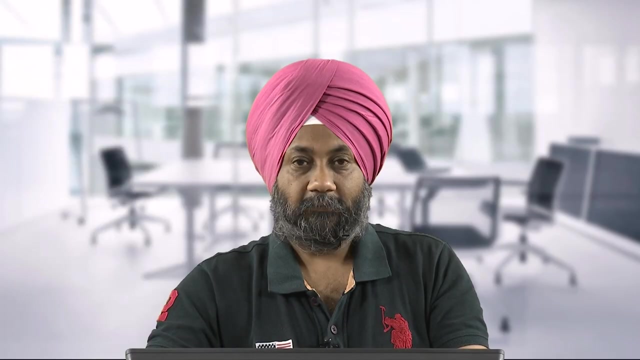 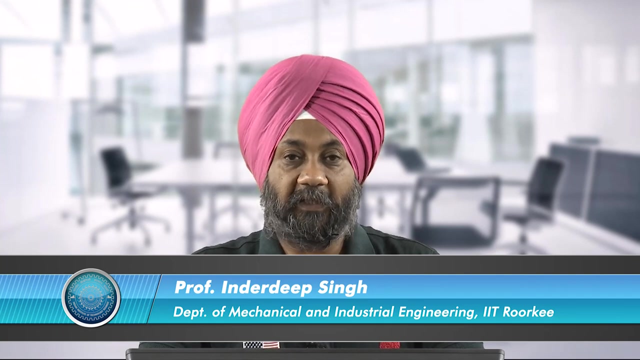 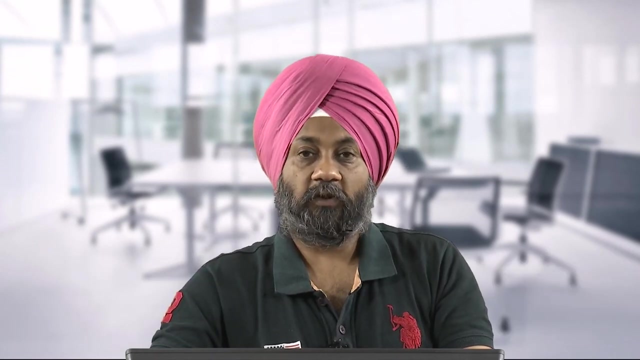 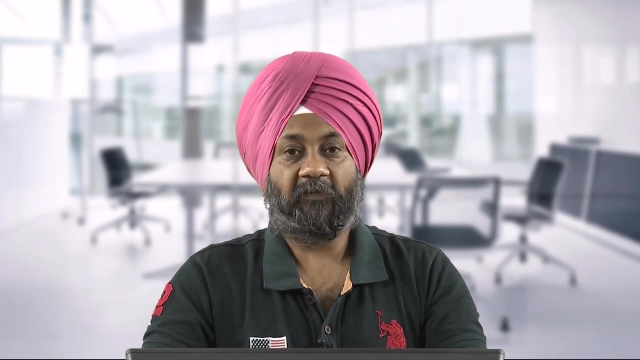 Namashkar friends, welcome to the second week of discussion in our course on manufacturing guidelines for product design. As you are well aware that in the last week our focus was on the manufacturing processes. We have tried to understand, we have tried to highlight, we have tried to discuss the 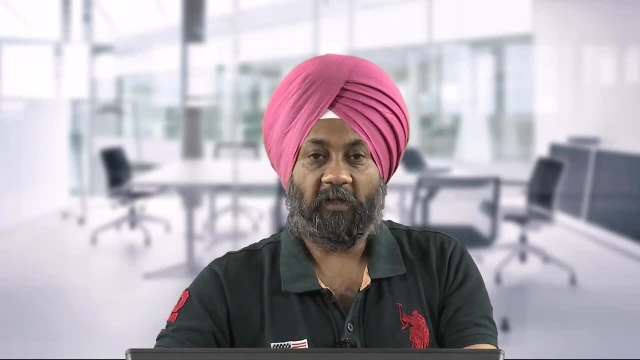 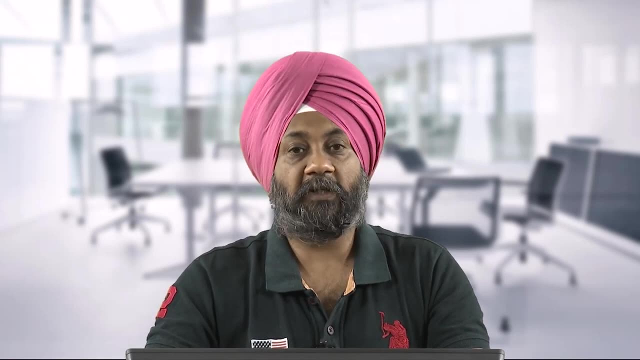 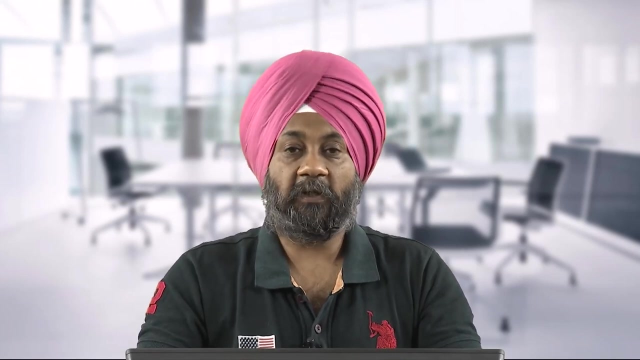 basic aspects of manufacturing processes. We have tried to classify the manufacturing processes, we have tried to understand the process capabilities of the most commonly used manufacturing processes And then we have tried to see that what are application areas or what are the typical applications for the various manufacturing processes. 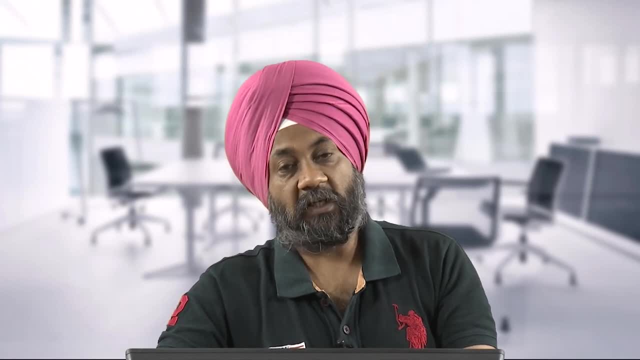 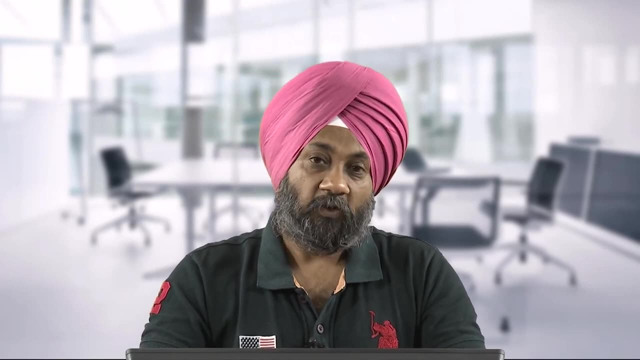 We have seen that wear casting can be used. we have seen wear injection molding can be used. we have seen wear blow molding can be used. So it was just to touch the tip of the iceberg, because the manufacturing is a very, very, very, very, very very. 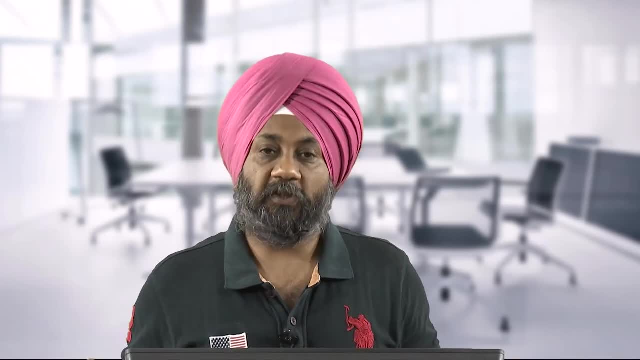 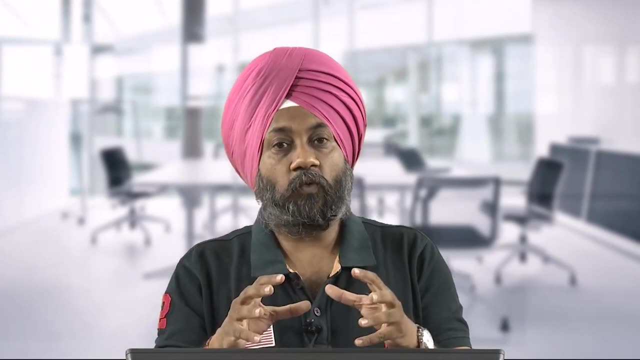 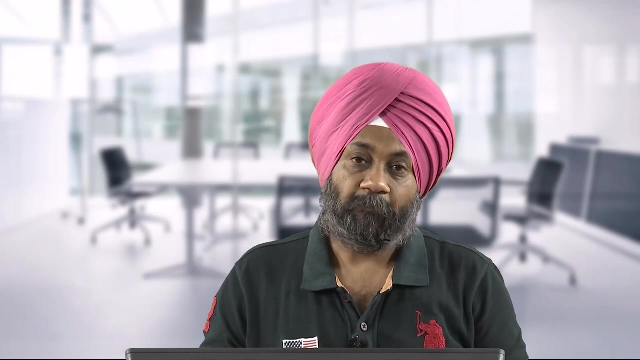 Diverse field with lot many processes that are used for manufacturing of different types of products. So we have just tried to understand that, if we want to understand a manufacturing process, what should be our focus? Now the focus can also be different as a manufacturing engineer, or as a production engineer, or as 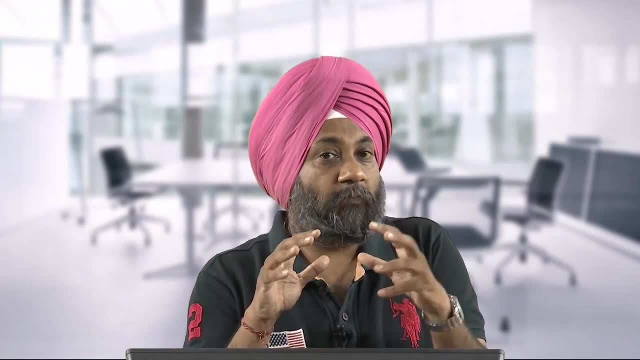 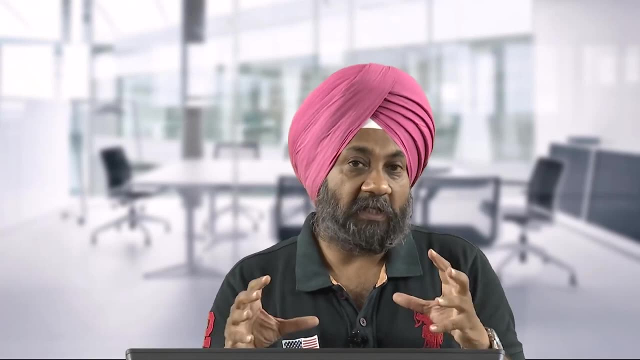 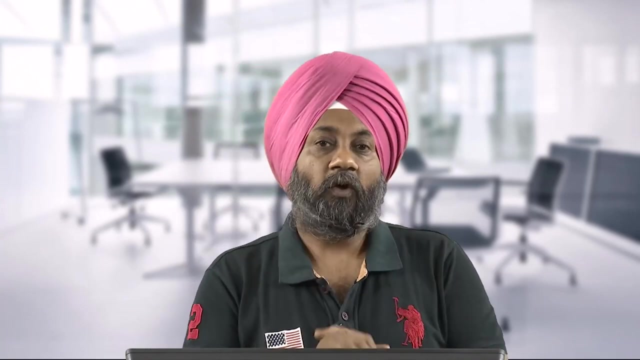 a mechanical engineer, I would like to understand the process in a much better, in a much deeper, in a much exhaustive manner, whereas as a product designer I would like to focus only on the applicability, only on the versatility of the process I may not be too much interested into. 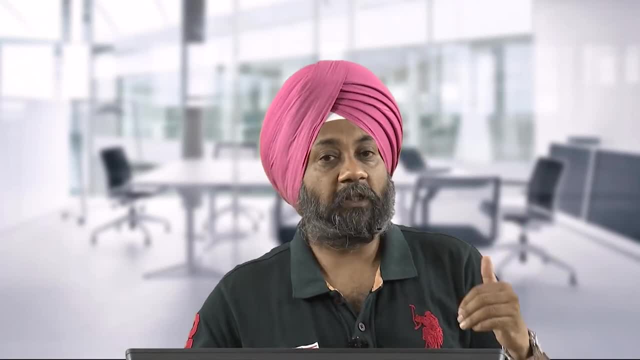 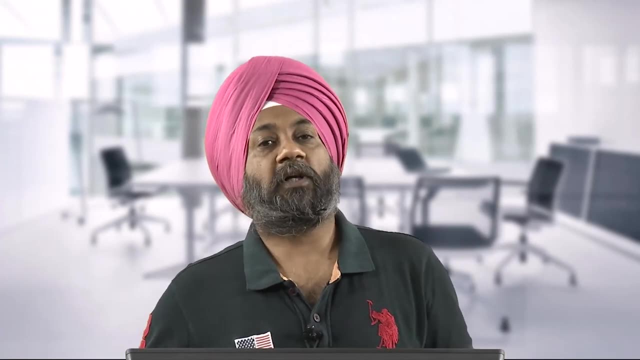 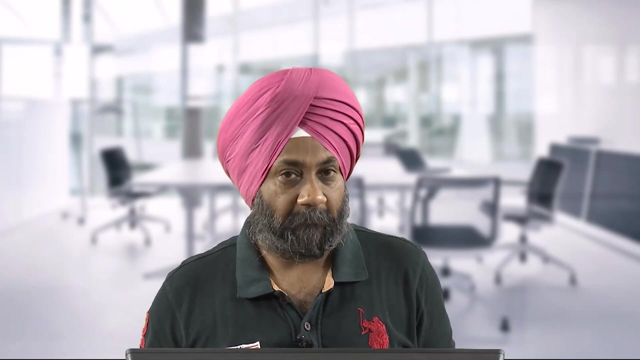 the process parameters or the process mechanism or the process mechanics. I will be only interested in what this process can do for me as a product designer. for example, suppose I have to make a very bulky product. it has to be made in metal. as a product designer, 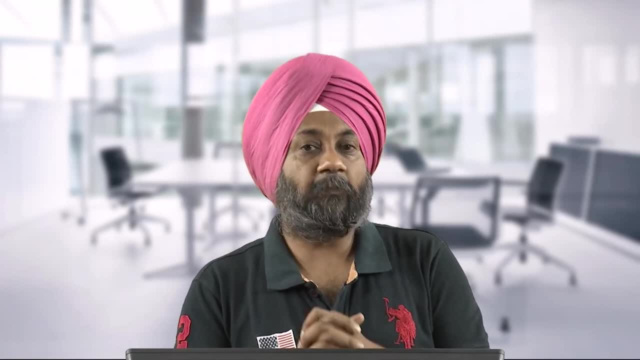 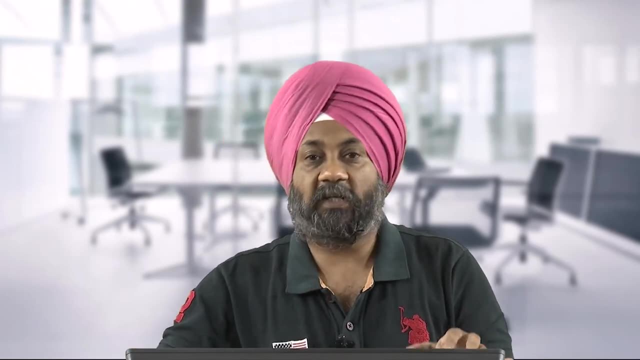 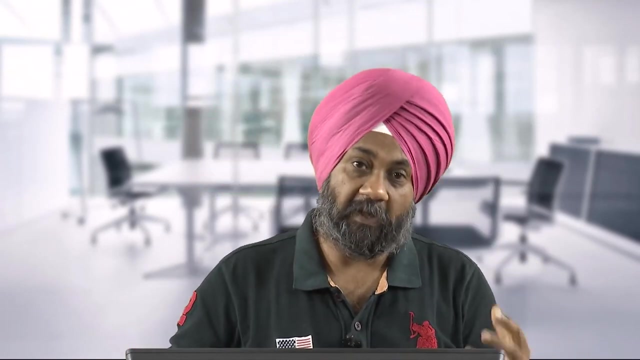 I will be interested to find out which process can help me to produce this product, And I may zero down on casting. that casting is a process which can give me bulky, large metallic products. Now the further design of the manufacturing process for making this casting, which is large. 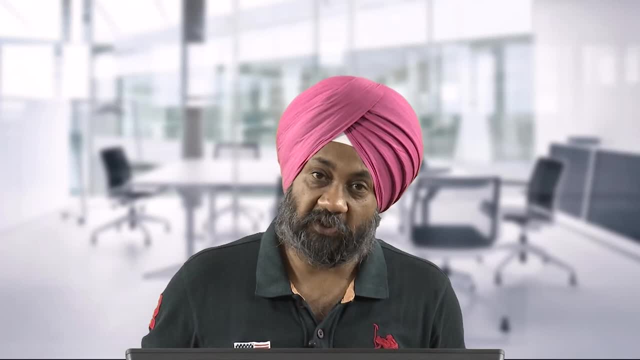 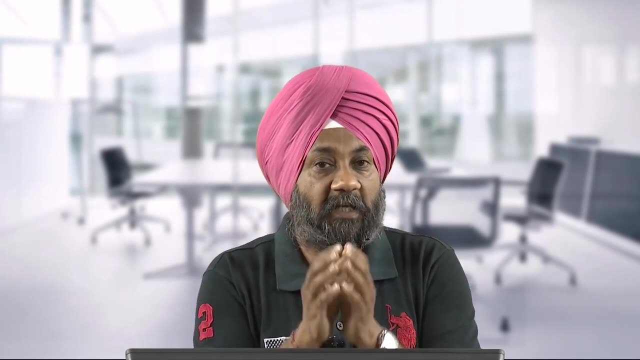 in size depends upon the expertise of the manufacturing industry. If you have any questions about it, please comment below. engineer or the mechanical engineer. But as a product designer, when I am designing the product, I must have some basic idea about how the product is going to be manufactured. 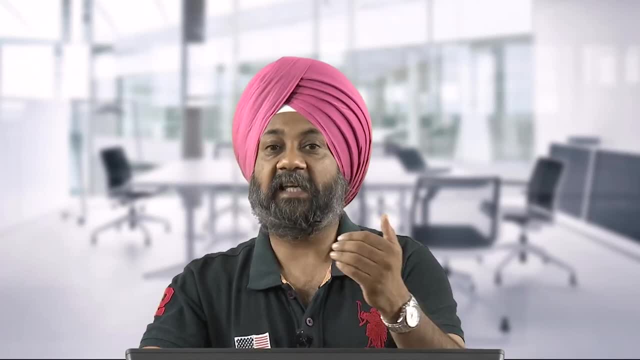 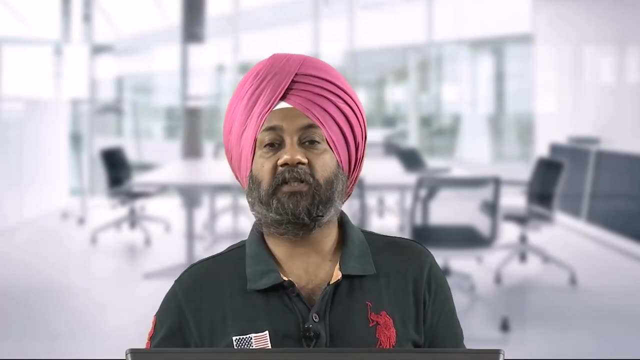 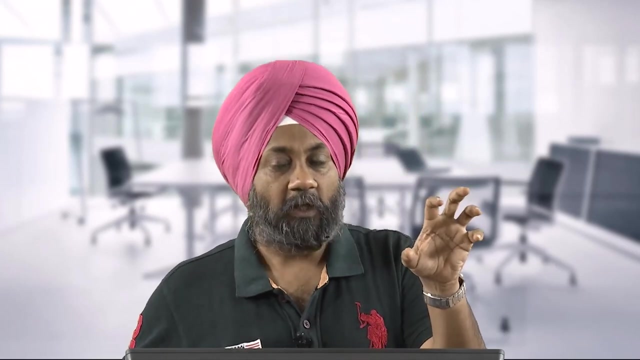 So if I have that idea, I can definitely liaison with a manufacturing engineer and try to fine tune that design in consultation with him. So therefore, we need to have basic understanding of manufacturing from the product designer point of view, and this course is designed for that purpose only. 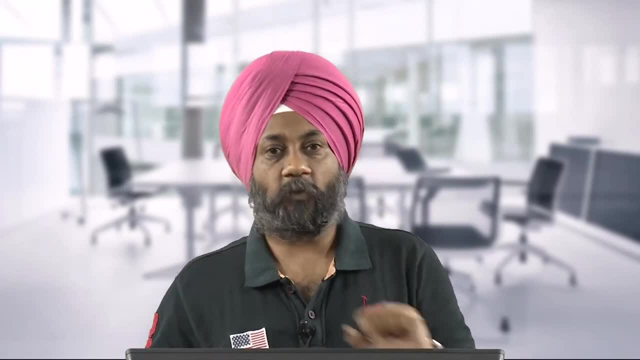 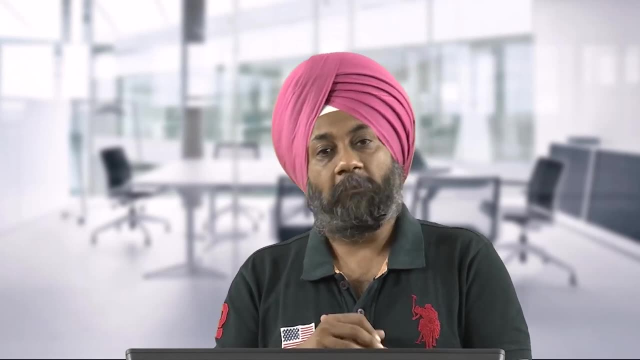 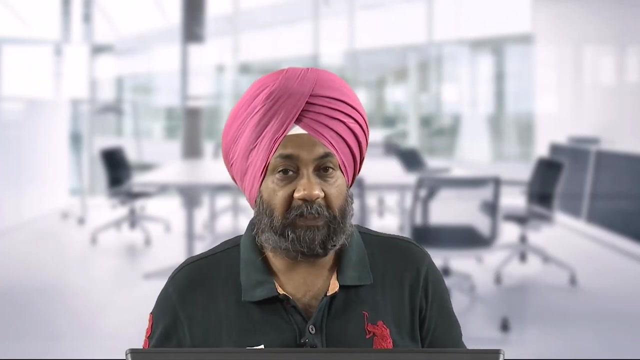 In the first week we had a discussion on the manufacturing processes. in the current week, that is, week number 2, our primary focus will be on the engineering materials because, as a product designer, we must know, we must have the basic understanding about the materials which we are going to use. 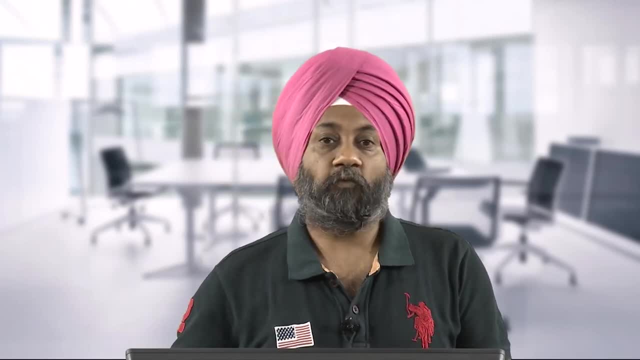 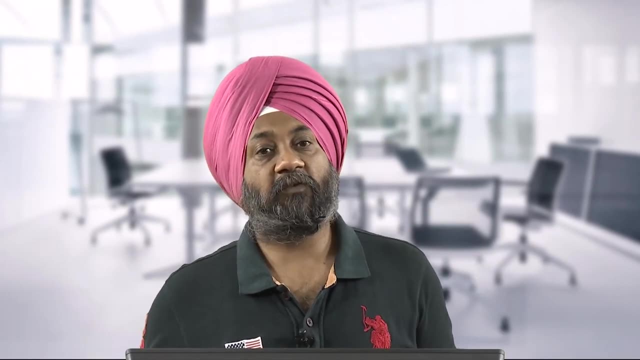 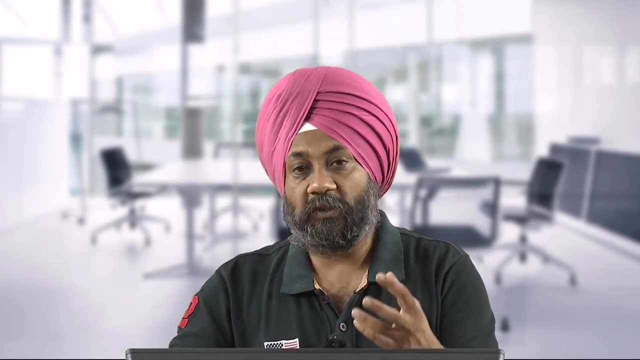 For fabricating our products. if we take the example of this recording studio, we can see there are different types of products that we are using in this studio, and each product is made by materials. So how much importance do we give to materials as engineers, or as managers, or as professionals? 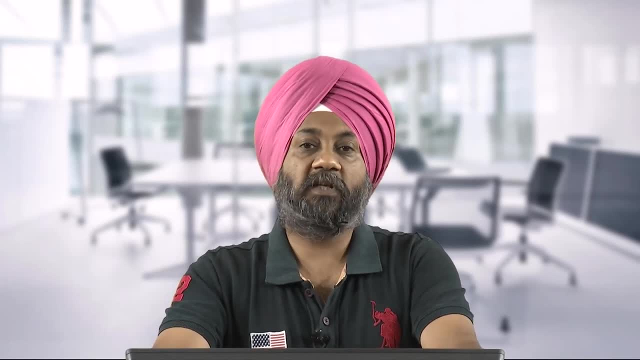 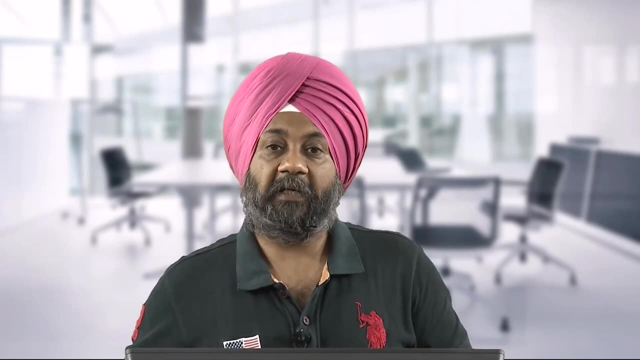 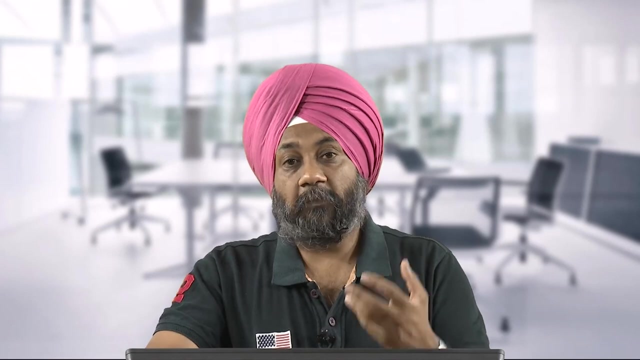 Most of the time, we do not give much importance to the engineering materials as well as the manufacturing processes. Let me take an example. when we get up early in the morning, we go to the washroom and brush our teeth. How many of us will be able to tell that? what is the material of the handle of the brush? 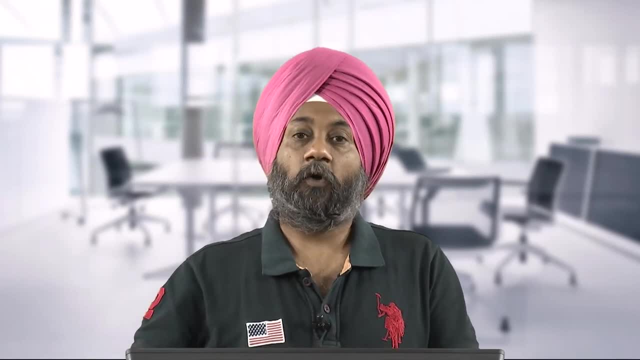 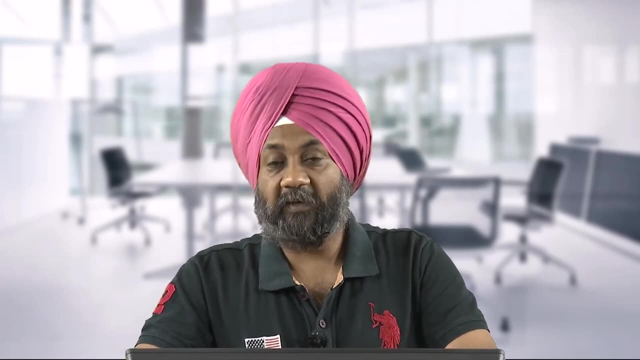 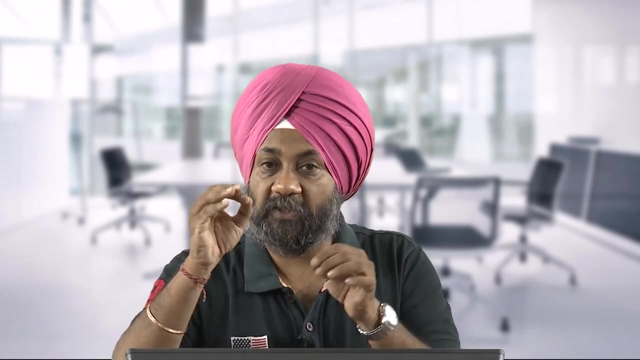 Many of us may not be able to answer this question. despite of our engineering degrees, despite of our management degrees, Many of us who have studied mechanical engineering, Many of us may not be able to name the process which is used for fixing up the bristles on. 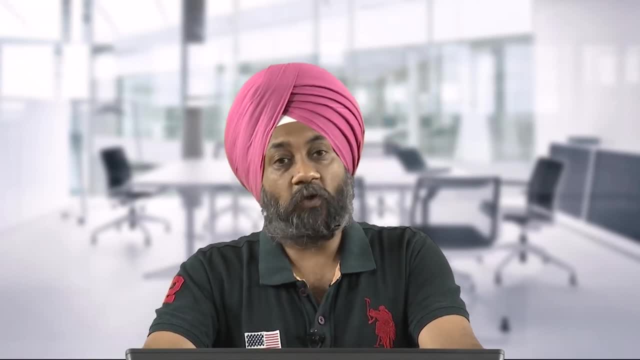 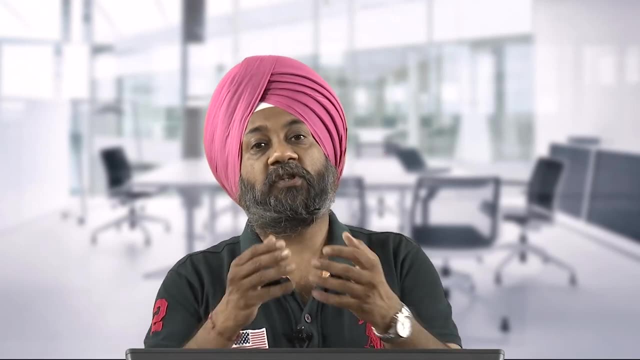 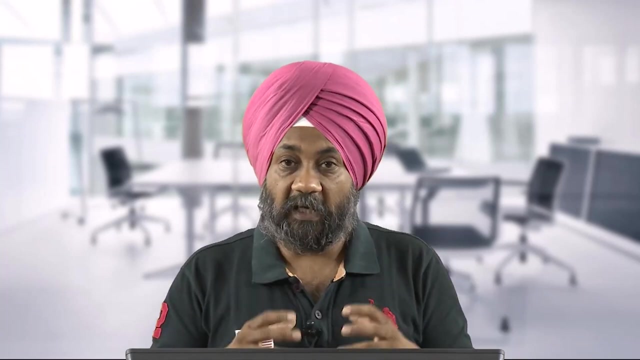 the handle of the toothbrush. So we do not give much importance to manufacturing, we do not give much importance to the materials which we see all around us. So, as a product designer, it becomes important for me to understand that. what are the various types of materials? 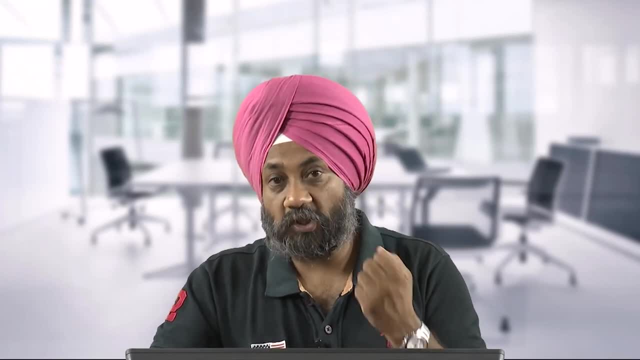 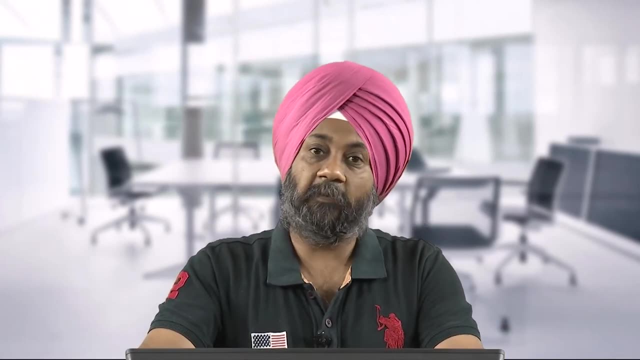 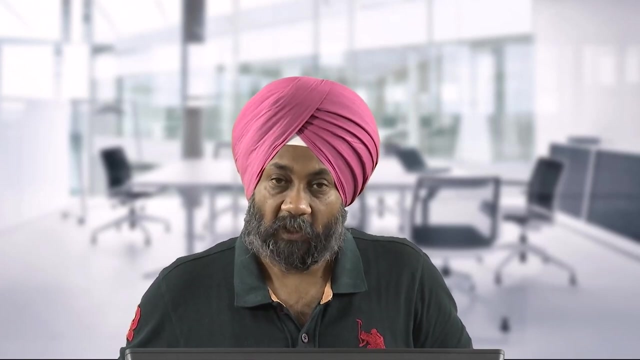 What are the specific advantages? What are the advantages- Application areas, limitations, exceptions- of the engineering materials and if I know that I will be able to make a judicious choice of material for my product design. Let us take an example of a chair. 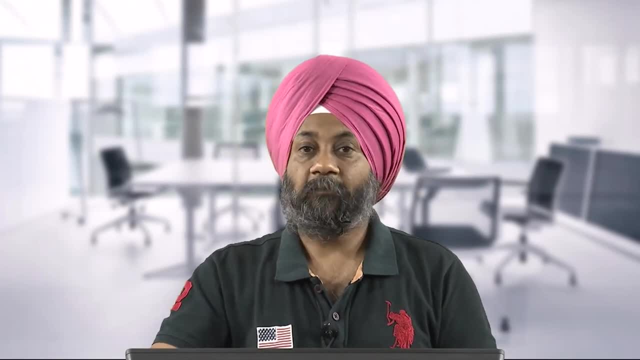 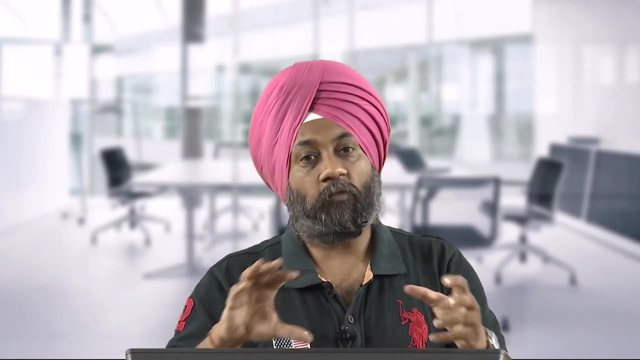 Now we can have a chair which is made by a plastic material. We can have a chair which is made by wood. We can have a chair which is made by metal. So we have different types of chairs made by different types of engineering materials. 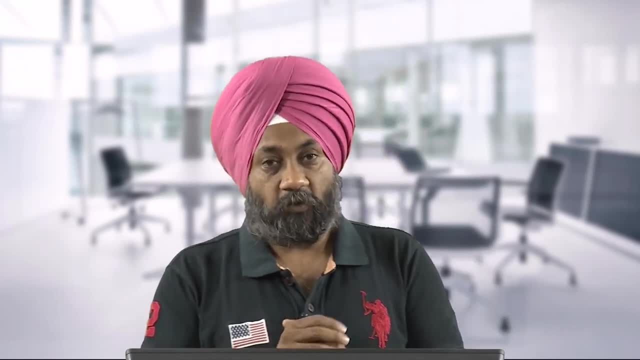 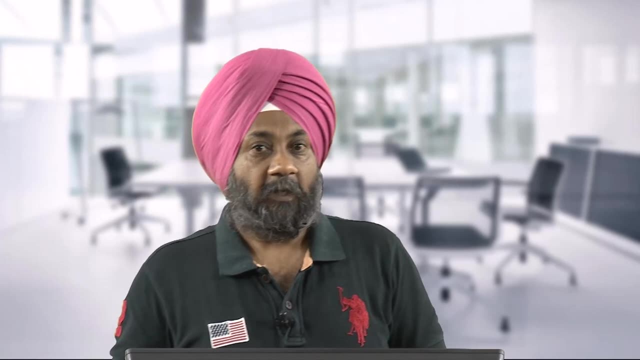 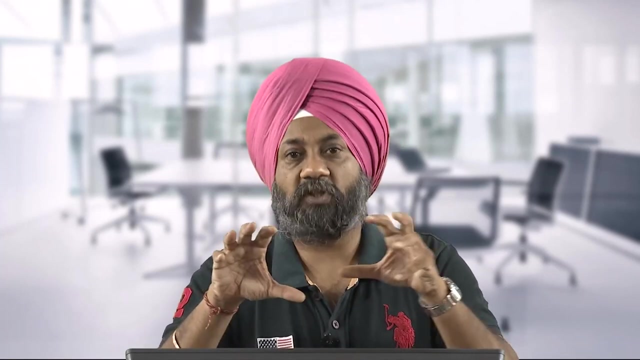 Now how this selection of material has taken place. So some thought process must have gone into this selection process, that where the wooden chair is better, where the plastic chair is better, where the metallic chair is better. So 3 different, the functional requirements remain the same: the functional requirement. 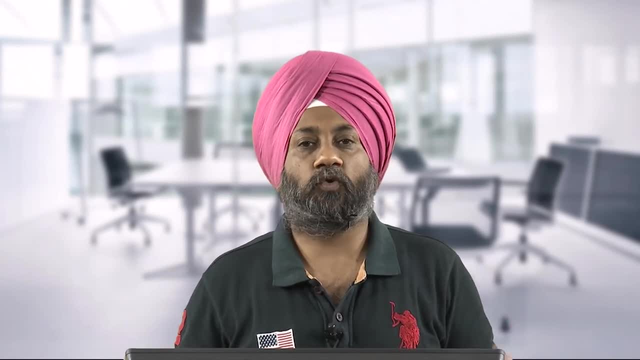 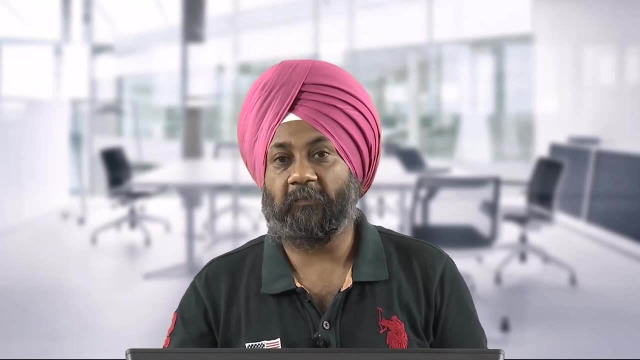 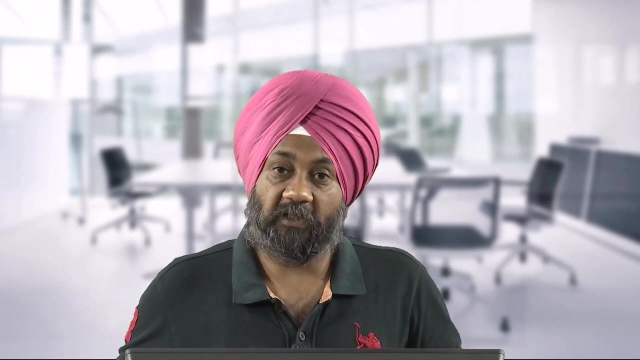 is that we have to provide a seat for a person, For a person who wants to use this product. but there are other requirements, or secondary requirements or tertiary requirements, which will definitely affect the choice of the material. For example, we want to design a chair which we have to move from one place to another. 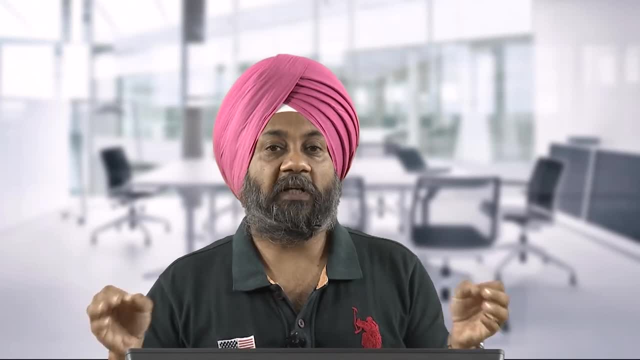 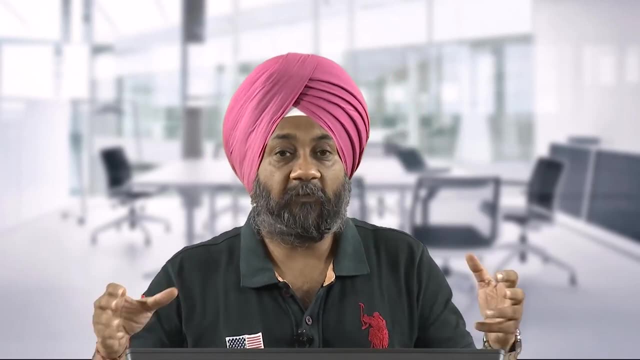 place on a regular basis, The most important requirement will be that it must be light in weight, because it has to be moved from one place to another place on a regular basis. Then we have to see that which material we must choose so that we are able to transfer. 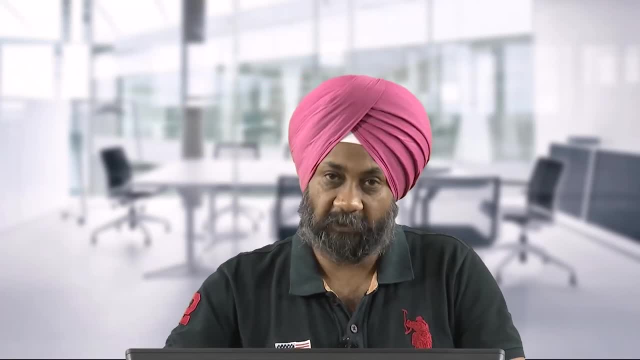 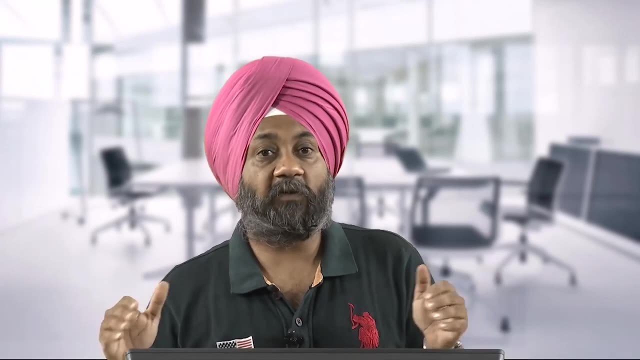 or transport this chair from one place to another place without much effort. On the other hand, we may like to fix the chairs at one place only and we do not want to move them in that case, but we want the long life because it is a permanent structure that we 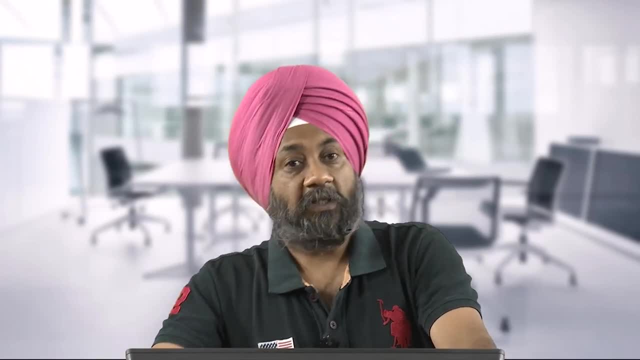 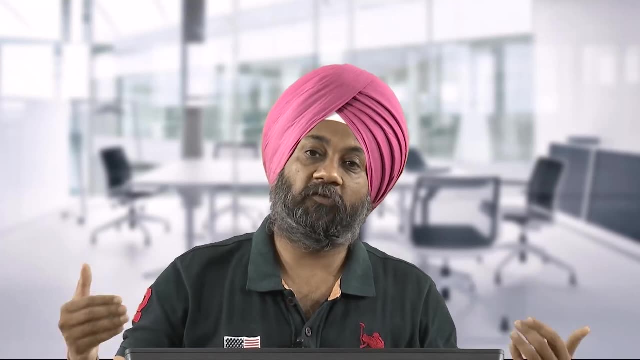 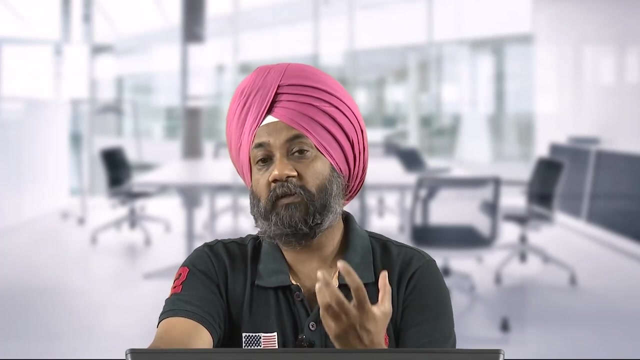 are creating, or a permanent facility that we are creating, So the chair need not be moved. in that case we need more strength, more life, So in that case the choice of material will be different. So therefore, as a product designer, I must have understanding about the various engineering. 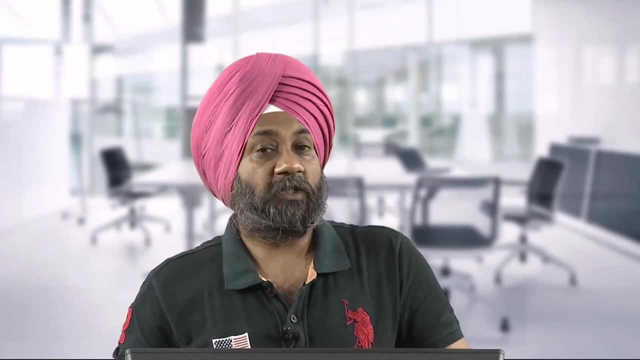 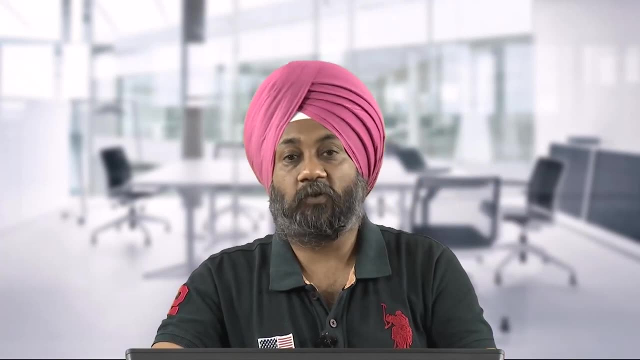 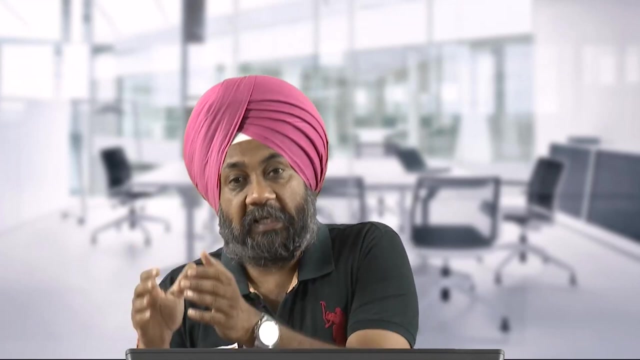 materials, the possibilities that exist, the classification of the engineering materials, certain examples we can take that in these situations these materials are used. And certainly when we advise, when we advocate, when we propose that this material can be replaced by a new material, we have to justify that, how the new material is used. 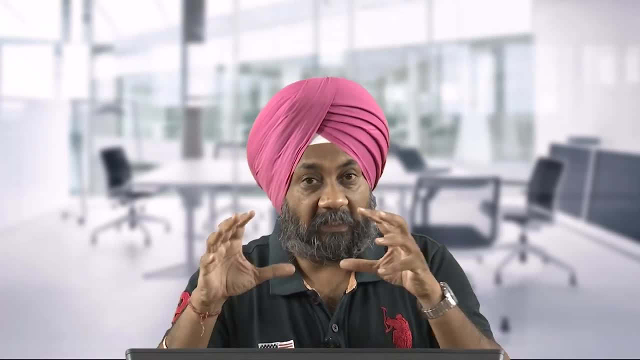 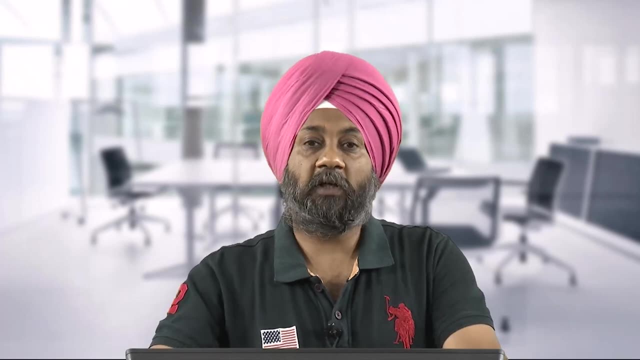 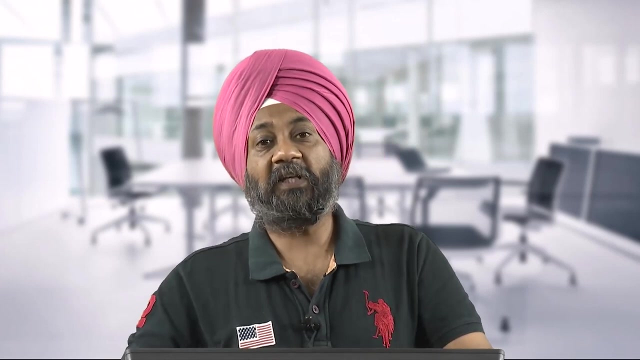 How the new material is better than the existing material. So all that kind of understanding a product designer must have in order to propose the use of materials for his or her product. So whenever the product design is being finalized, as a necessary requirement we have to specify: 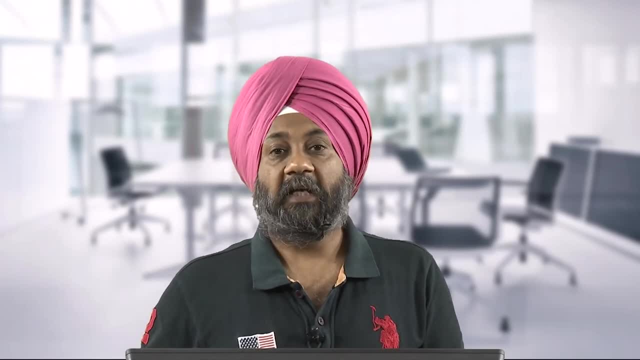 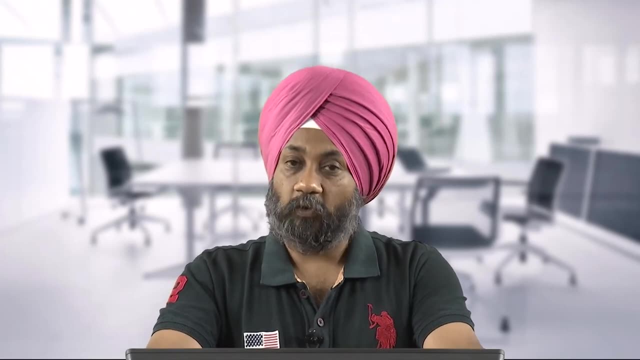 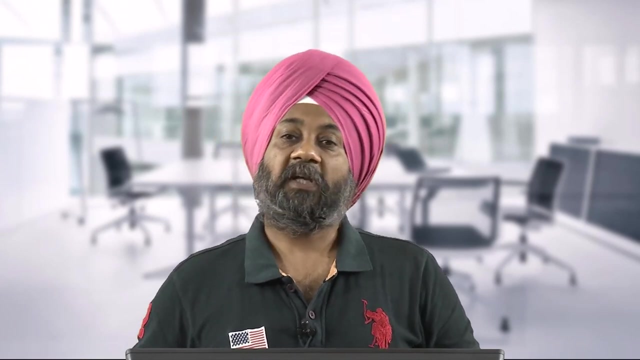 that this product will be made, by which material, and what are the various types of engineering materials that we are going to study, that we are going to discuss In today's session, with certain examples. So let us now start our discussion. The title for today is engineering materials. 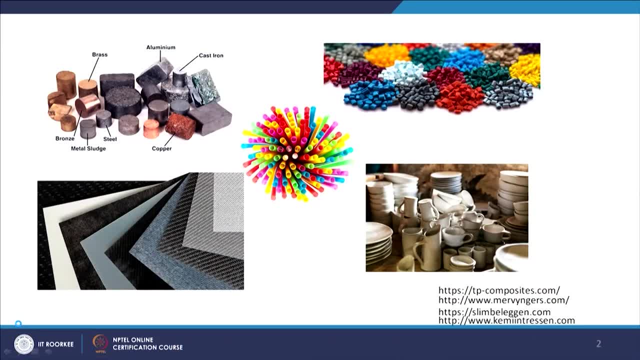 Now on your screen you can see different classes or different types of engineering materials. The first category that we have highlighted here are the metals or the alloys. You can see it is clearly written. the names are given metals or alloys. So you can see here aluminium, brass, cast iron, copper, steel, bronze, metal sludge. 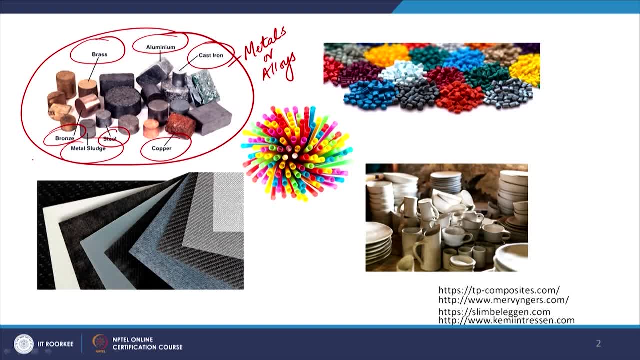 So all these fall under the category of metals or alloys. All these are the polymer pellets and also we can call them in the general name as the plastics. These are some of the plastic products which are shown here which are made by these colored pellets. 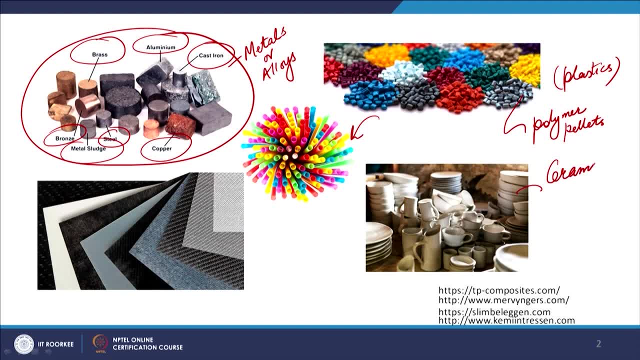 Then this is another category of engineering materials that we call as the ceramics. So we have plastics or polymers, we have ceramics, we have metals or alloys, and then we can have a category of materials, which we call as the composites, specifically used for specific 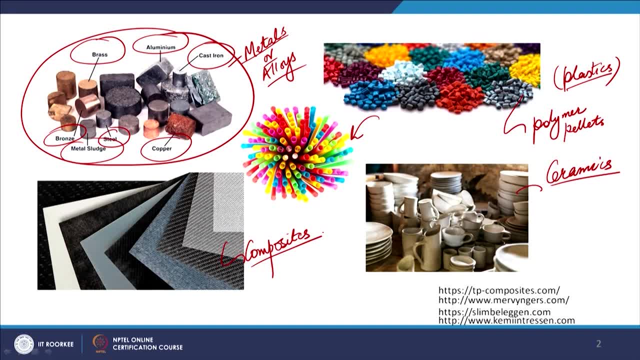 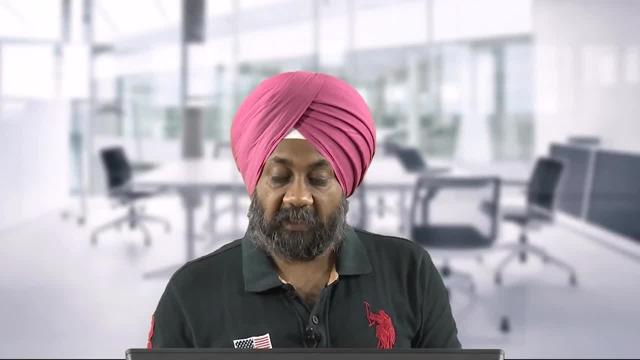 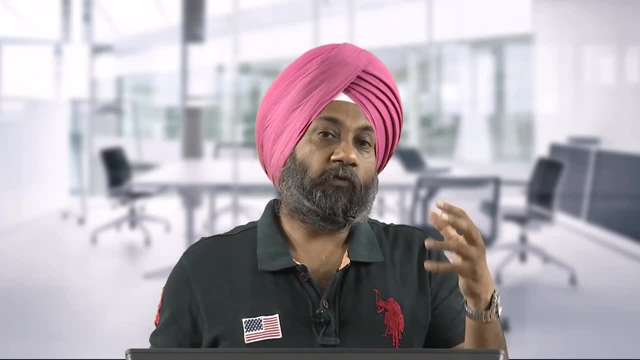 requirements, light weight requirements, High temperature requirement. depending upon the type of the composite material, we can have different types of application areas. So here we can see 4 broad classes, 4 broad families of engineering materials. So if you talk of metals, we can discuss metals in a 20 hour session. 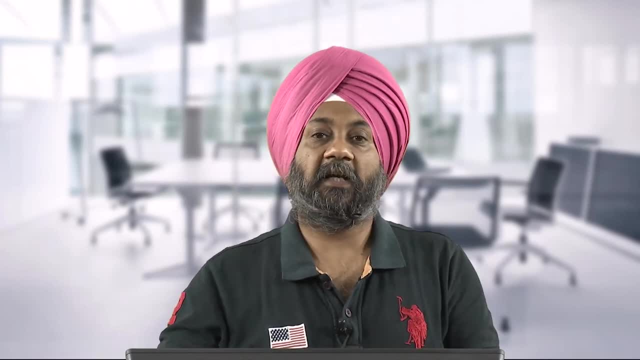 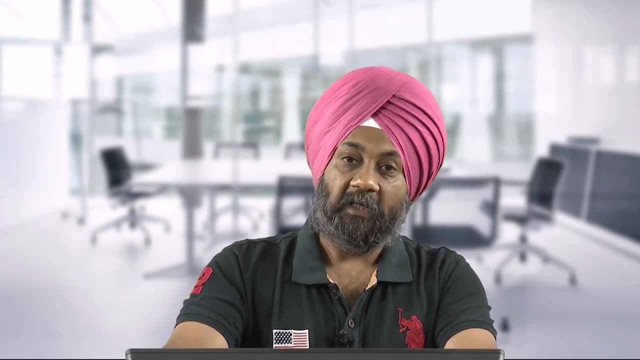 There are different types of courses regarding the metallurgical aspects of metals, the joining aspects of metals, Which are already available. So you can see that These are available on NPTEL. But from product design point of view, once we have to choose a material, we need to understand. 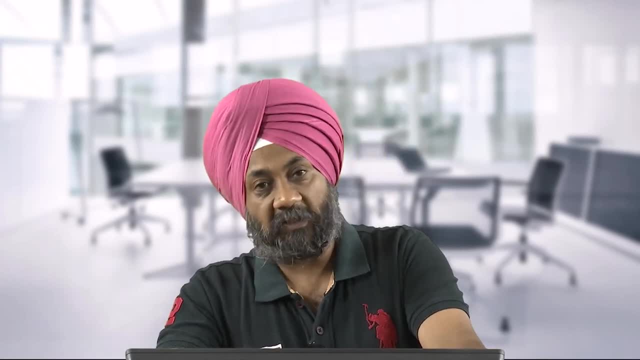 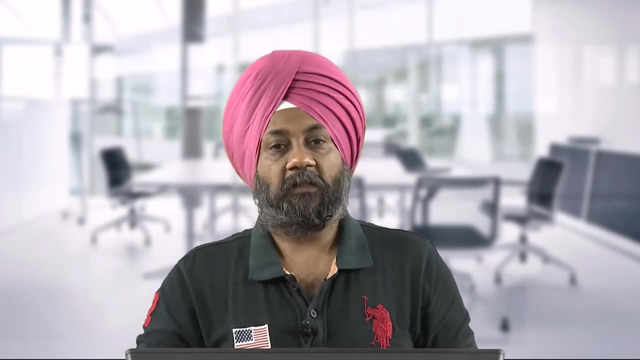 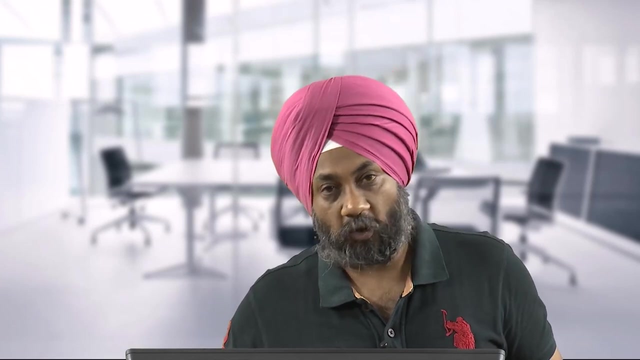 the basic characteristics of that material. that we will try to address maybe in the subsequent sessions in this week. So but today our target is to classify the engineering materials. So engineering materials: broadly we can see there are 4 families here: metals or alloys, polymers, ceramics and composites. 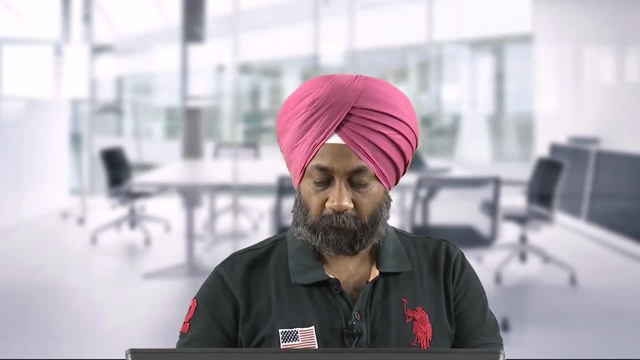 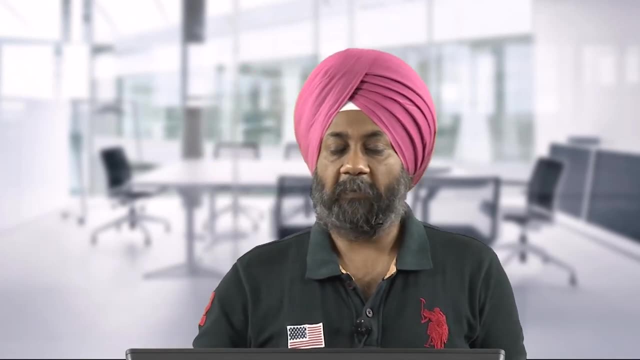 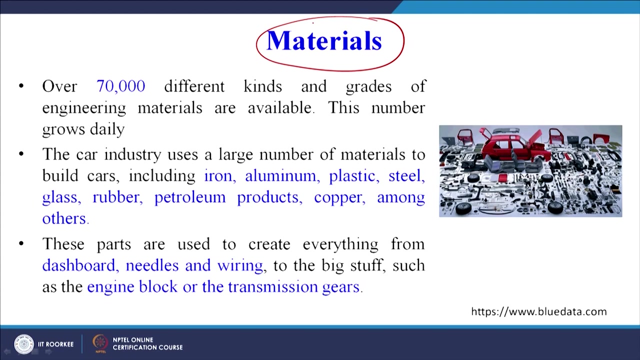 So let us now see how we can classify them. So we will come to the classification, But let us have a brief introduction about the importance of materials. So what is? we can say the depth and breadth, or we can say the length and breadth of the. 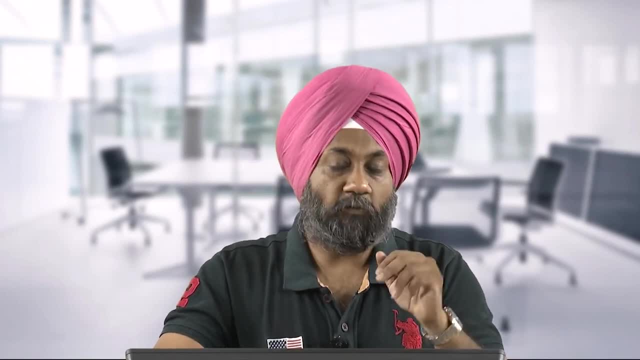 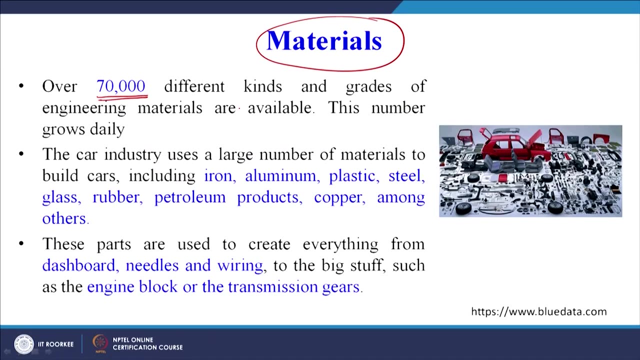 field of materials science and engineering. We can see from here over 70000.. 70000.. Development: 50,000 different kinds and grades of engineering materials are available And this number grows daily. And if you refer back to our first week of discussion, I think in the second session we 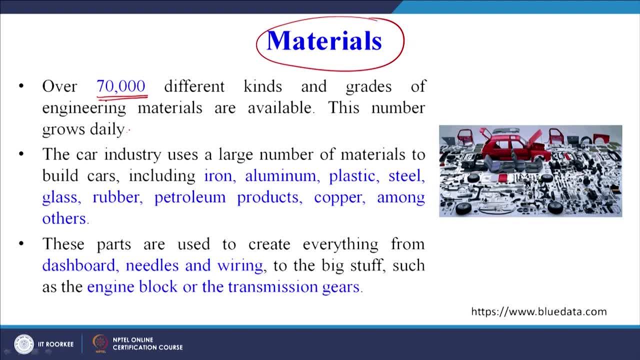 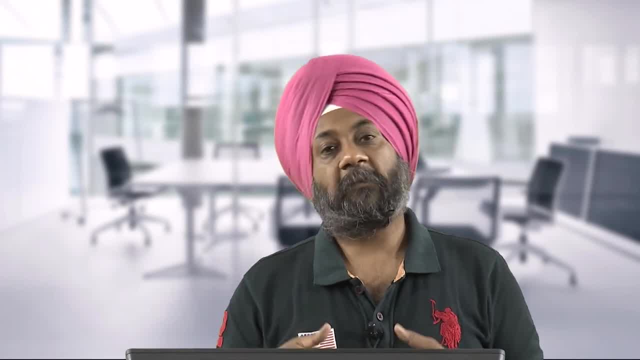 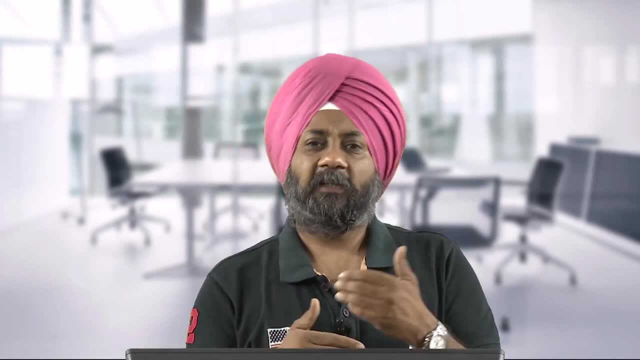 have seen that. why do we need to develop new and new manufacturing processes? Because the new and new materials are being developed every day, maybe every week and every year, Depending upon the specific applications. Every Day There is a discovery, scientific discovery or invention, whereas a new material or a combination 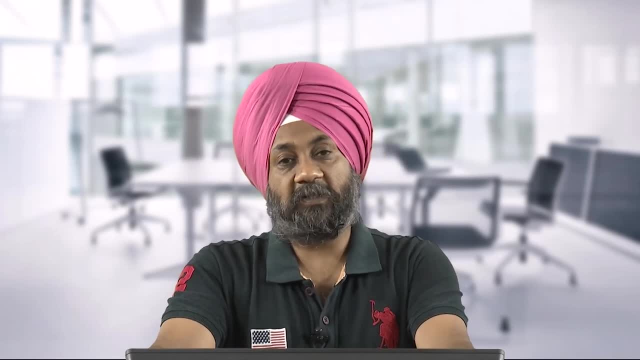 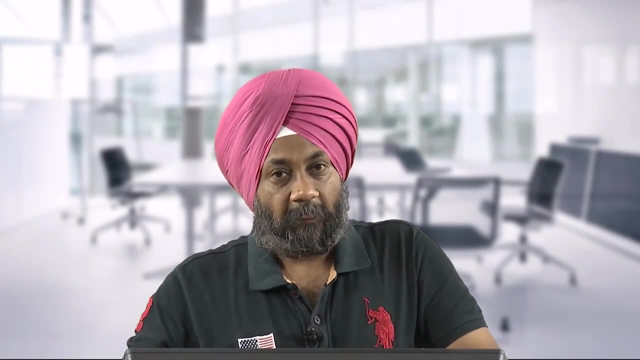 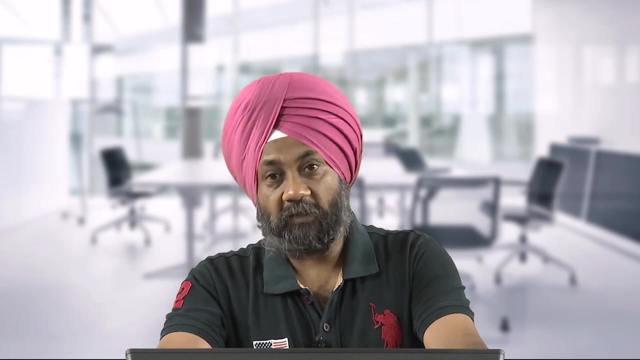 of materials is being developed to address a specific application. Just few days back, the environment day has passed And we have seen there was lot of focus about the use of plastic materials. So within this field, which is one specific family of the overall family of engineering, 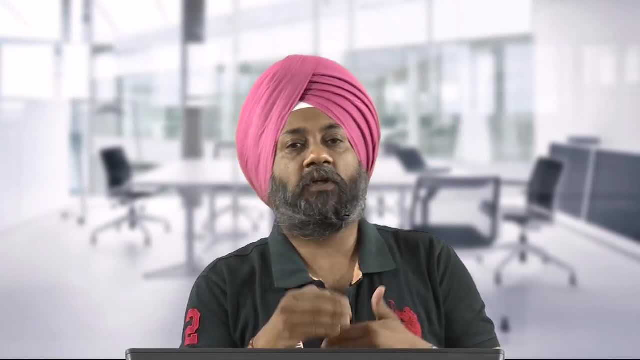 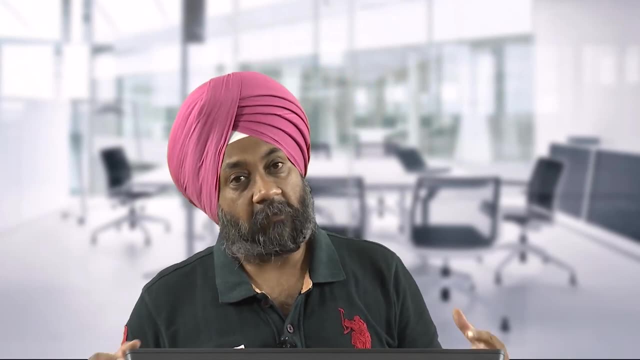 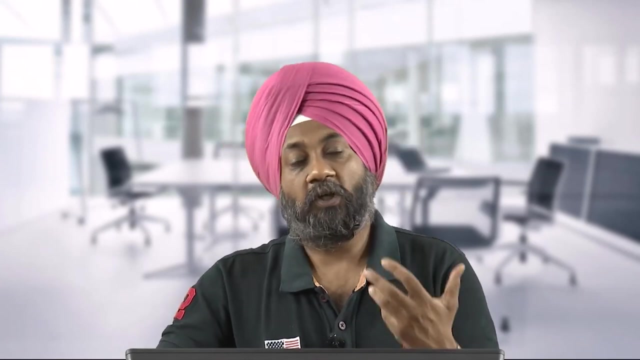 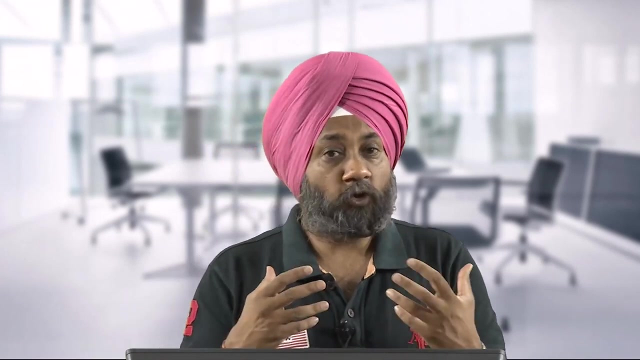 materials within plastics, there is lot of focus on developing new and new types of polymers which are biodegradable in nature, which are environment friendly in nature. Maybe every day, researchers are putting efforts and trying to develop materials which do not harm our environment, which are friendly to the environment, in which the philosophy can 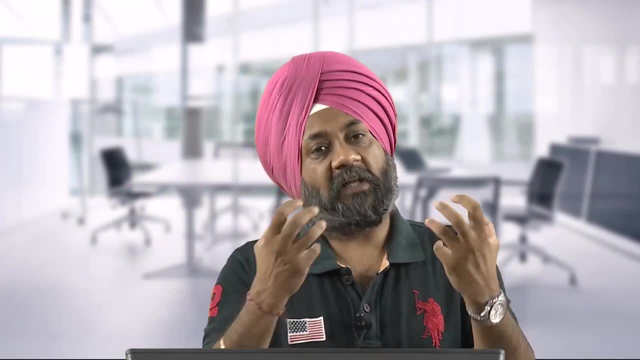 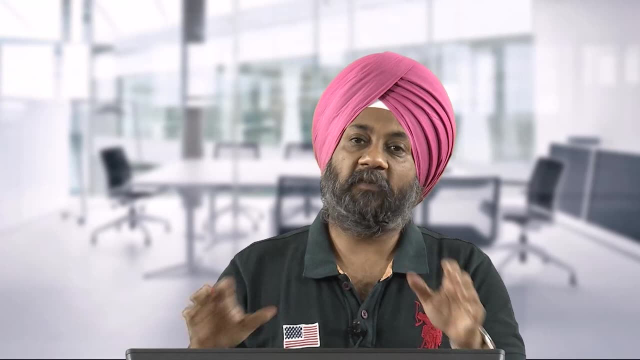 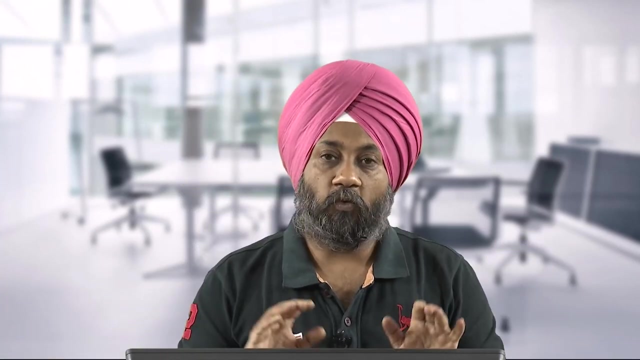 be that we derive certain raw material from our environment only And then make it a engineering material, make a product out of it and finally, once the product has lived its life, the material can be pushed back into the environment without causing any harm to the environment. 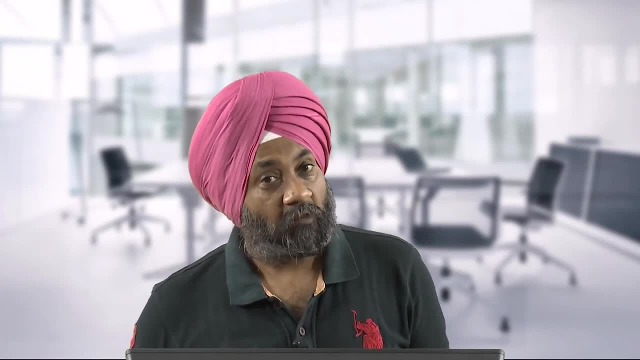 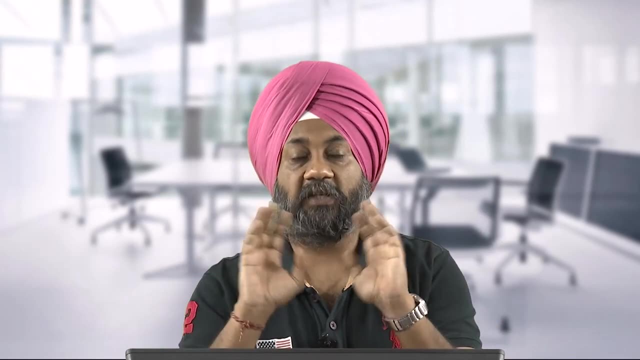 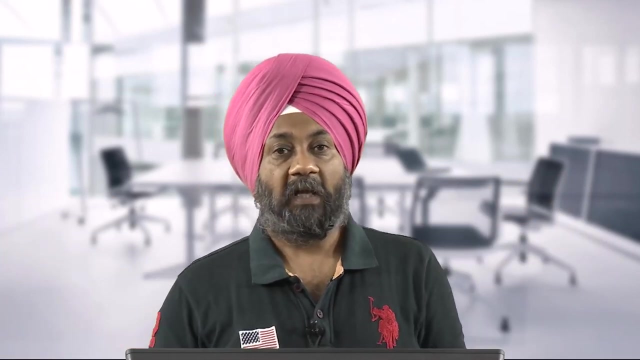 So that kind of philosophy is developing in which we are trying to harness the potential which is available in the materials which we see around us, in the environment, in our ecosystem. So we try to derive the raw materials from our ecosystem and then try to develop them. 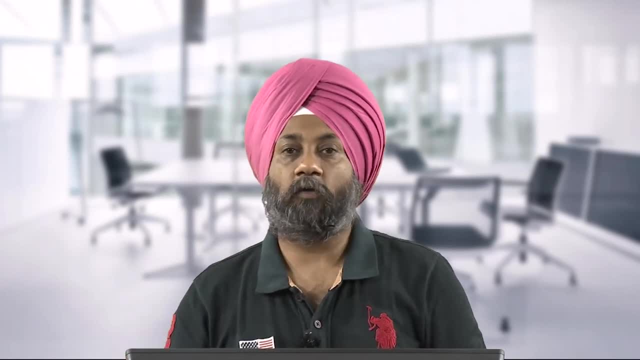 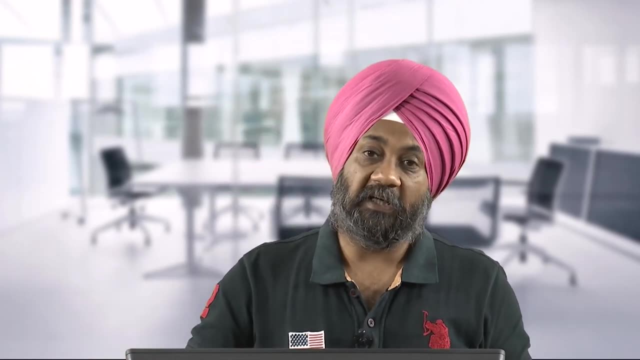 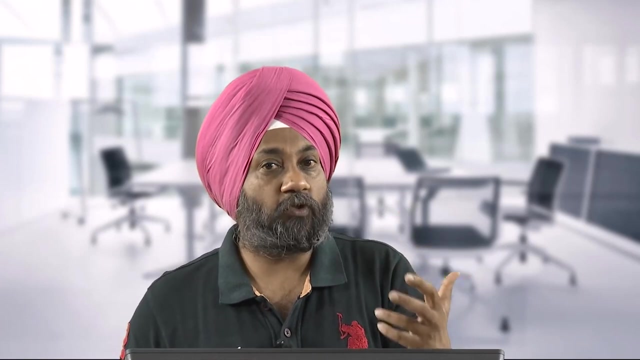 into engineering products and finally dispose them of into the environment in a much cleaner way. So new and new materials are being developed every day and therefore we need to understand, as a product designer, these advancements so that we propose the use of the materials which are friendly to the environment. 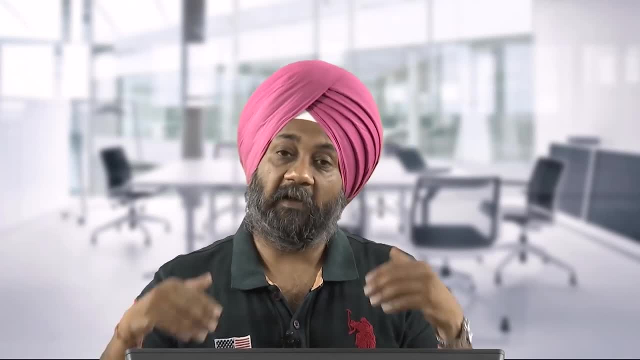 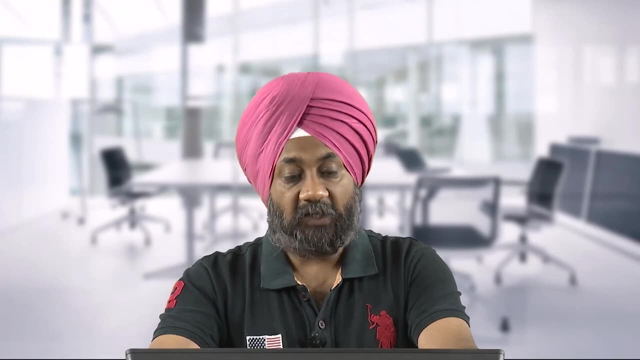 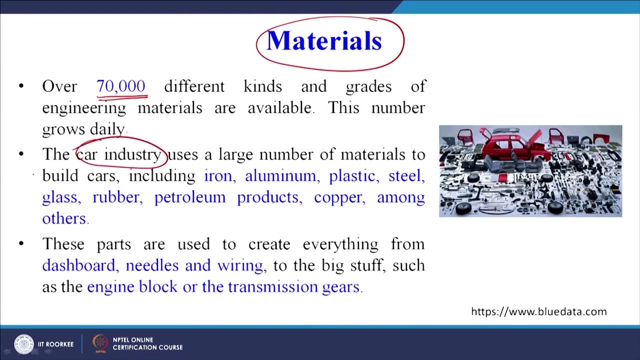 So 70,000 is not enough. 70,000 is not exhaustive number, so every day we may be finding that there is some new development in the field of materials science and engineering. So just to take one case, the car industry we have taken. the car industry uses a large number. 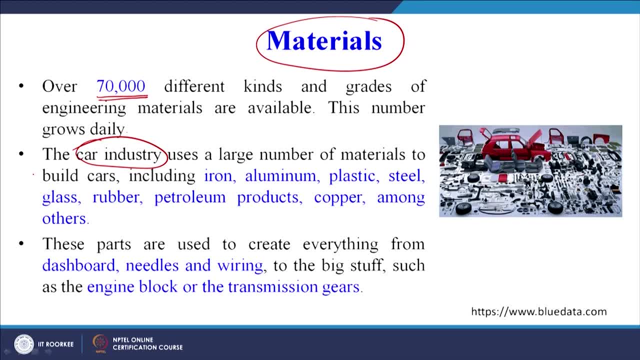 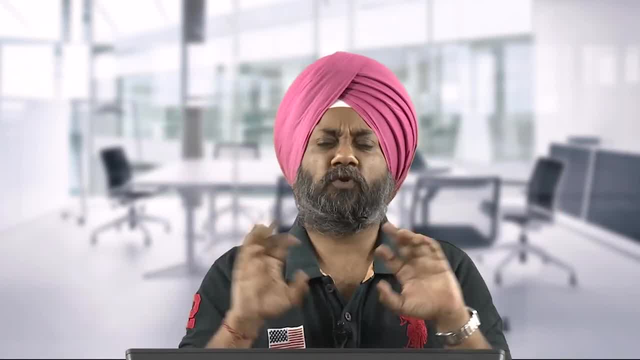 of materials. Now, what type of materials we see in the car. most of us may have used car or maybe driving in a automobile. If we see around, So, So many materials, are there? the seat that we are using, on which we sit, you see there. 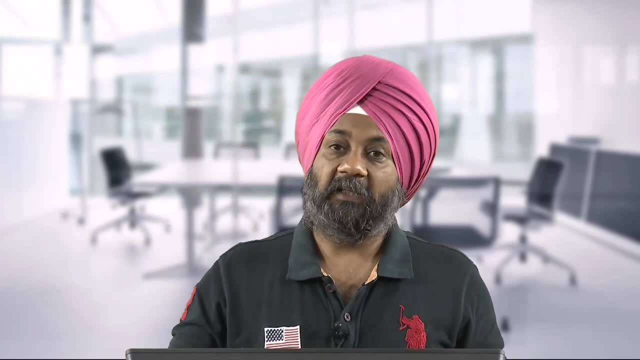 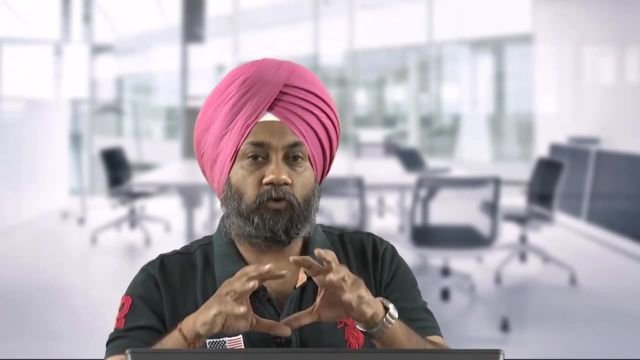 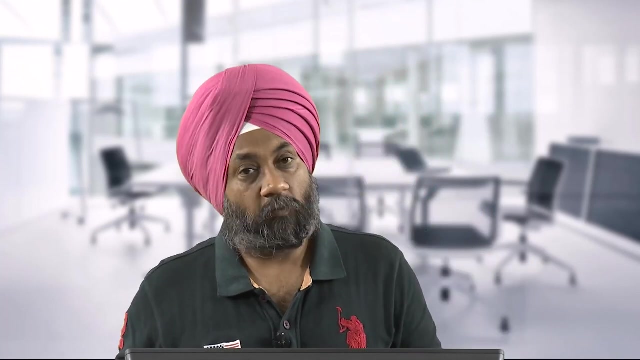 is a foam, which is a kind of a engineering material. the handle that we hold may be a metallic handle in the car or in the bus. So any automobile you take, so many engineering materials you see around, even if you are driving in a air, if you are travelling by air, in an aircraft. 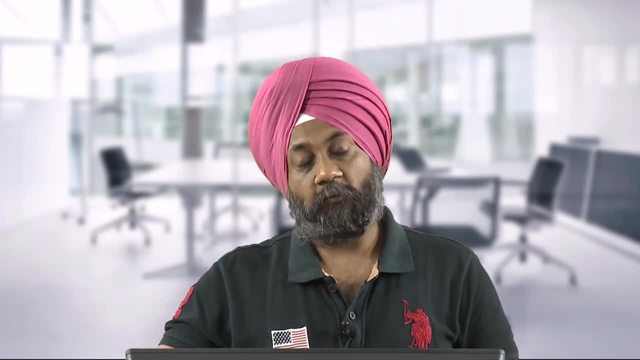 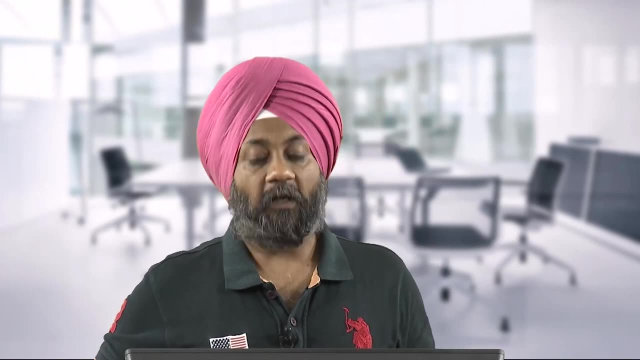 So many engineering materials you see around you. if you are travelling in a train again, you will see So many engineering materials around you. so in car also, it use the large number or materials which are use to build the cars. Now, what can be these materials? 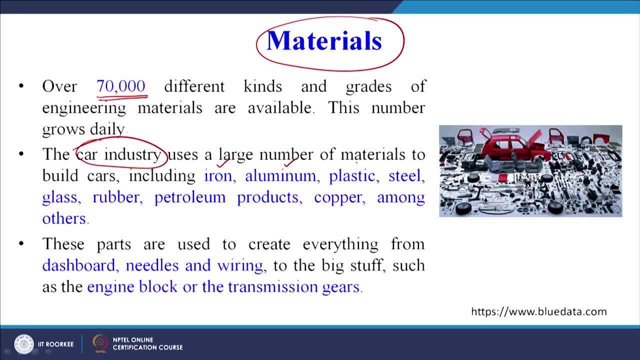 Let us see iron, alumini, plastic, steel, glass, rubber, petroleum products, different polymers, copper and among others. So we can see just a spectrum of materials Which are used for making the car. Now, when we are designing a product, we have to see that which material we must choose. 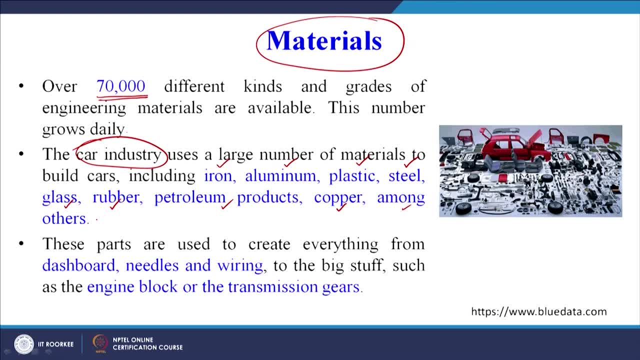 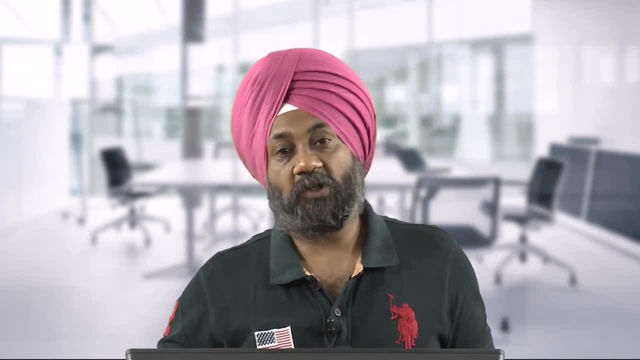 and large variety of materials are available with us. So these parts are used to create everything from dashboard needles and wiring, which are maybe our domestic applications, to the big stuff such as engine block or the transmission gear, which are engineering products. So we can see from the most simple part. I started the today's session with a very 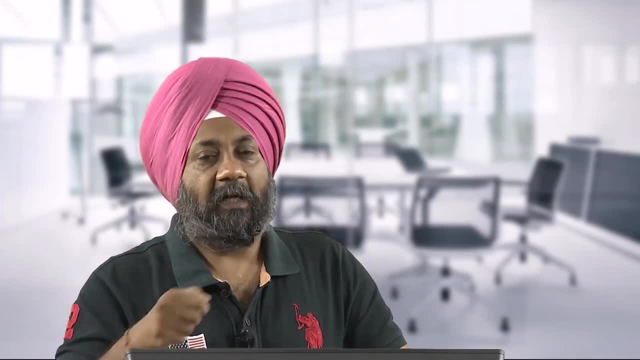 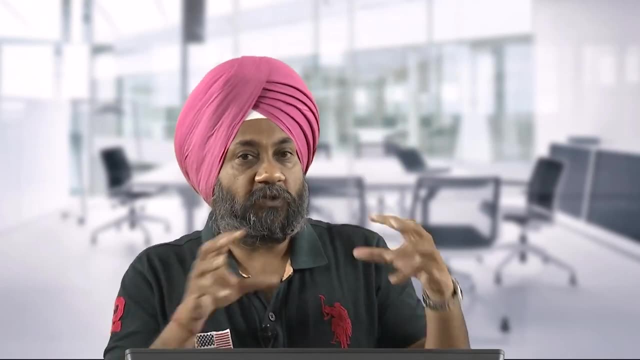 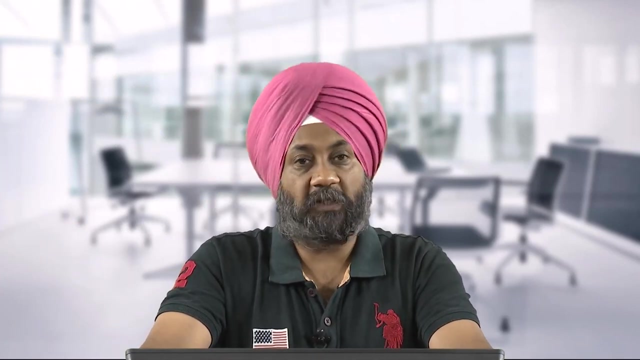 simple example of a toothbrush: a handle of a toothbrush and the bristles that are fixed on the handle to make it usable product. So from simplest product to the most sophisticated product, for example for aircraft applications or space craft applications, engineering materials find their applications everywhere and therefore 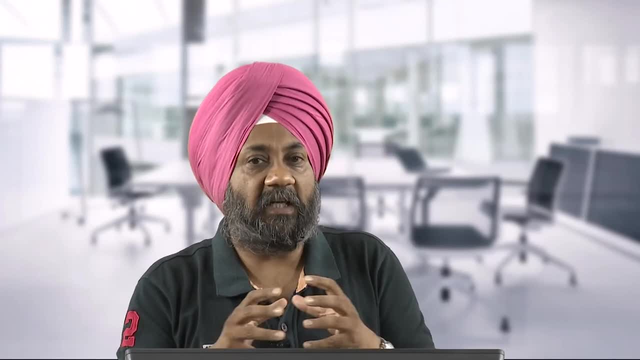 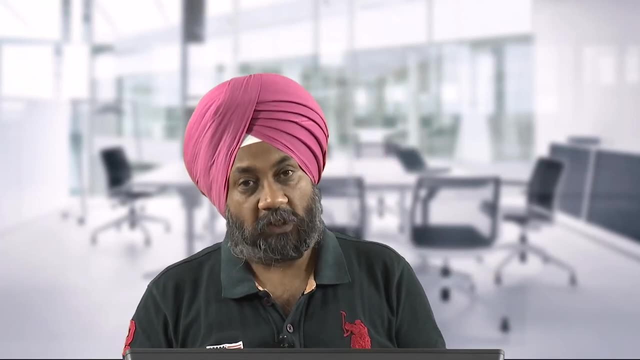 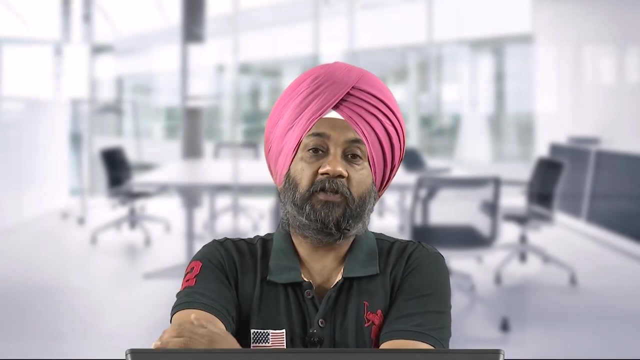 as a designer, I must have. So this is the basic understanding about the different types of materials that are available to be chosen, or from which we can choose what type of material is applicable for our product. Another example that I have taken today is of a chair. 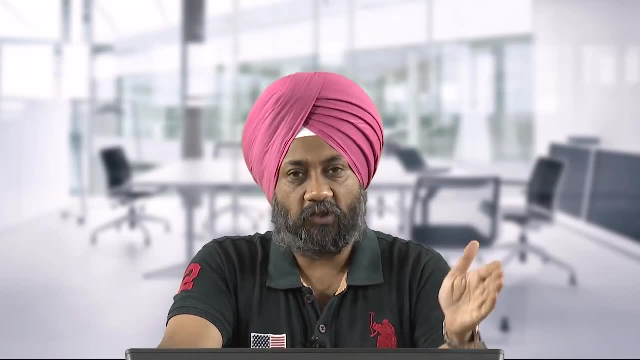 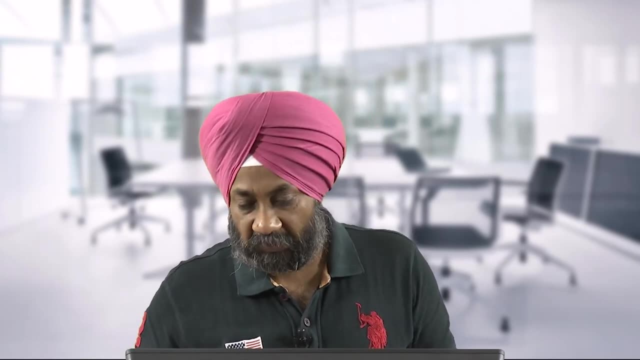 So we have seen that- 3 different- metallic chair, plastic chair, wooden chair. So depending upon the application, we will choose the material. Now what is the list that is available with us? so different types of engineering materials are available. So already we have seen the examples. 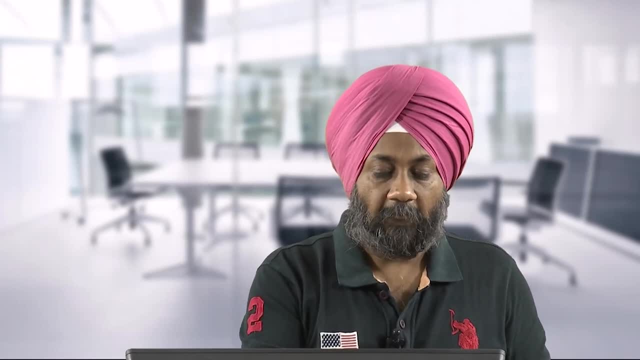 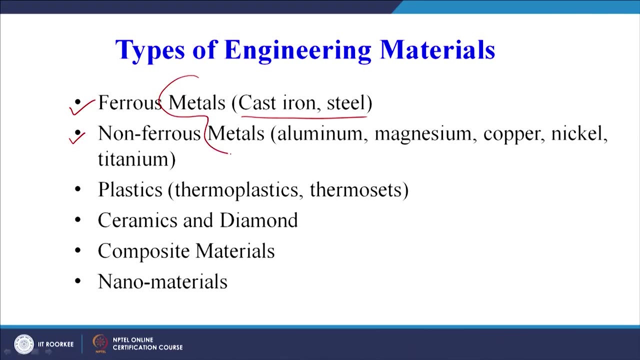 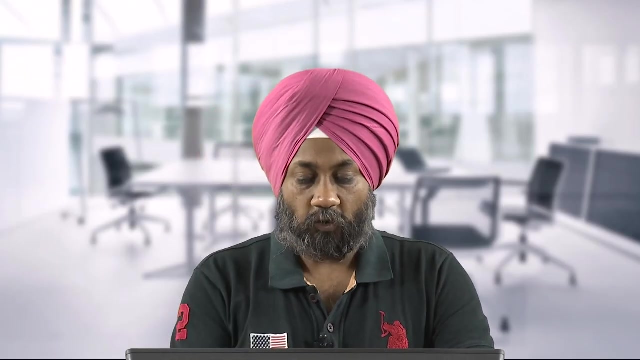 So now let us further classify them. We can have ferrous metals like cast iron or steel. we can have non-ferrous metals, So both are in the metals category only. but one category can be ferrous family, another can be non-ferrous family. 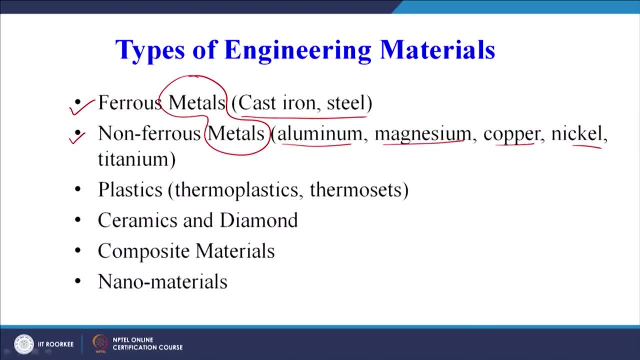 So we can have aluminium, magnesium, copper, nickel, titanium, So we can have non-ferrous metals. Then we can have plastics. Okay, Then we can have thermoplastics and thermosets, Then we can have ceramics. one category can further be diamond. 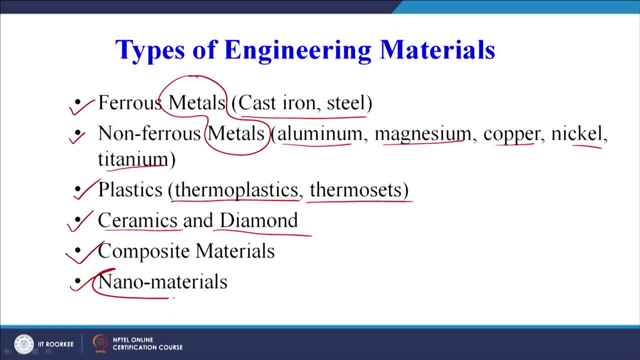 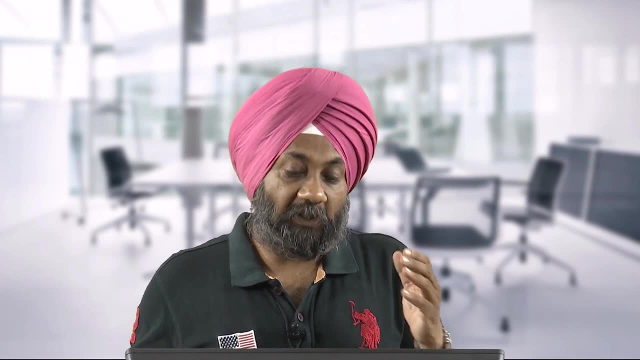 Then we can have composite materials. one category can be nanomaterials, So we can have nanomaterials coming out from any of the categories which are already mentioned. So major classification for engineering materials has been explained here. Now within this you can write some places. 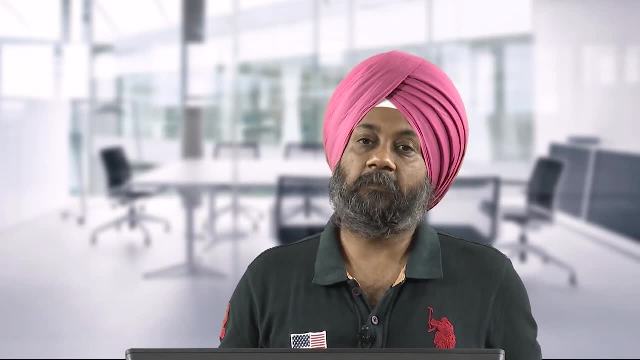 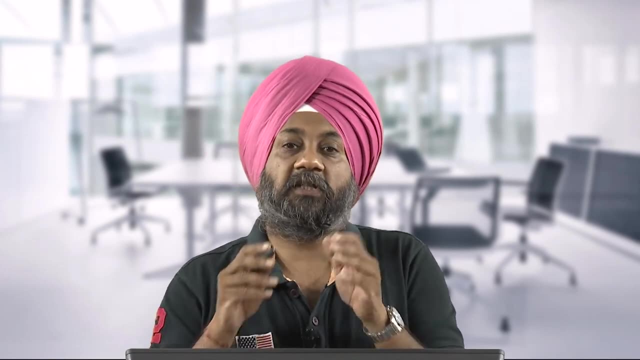 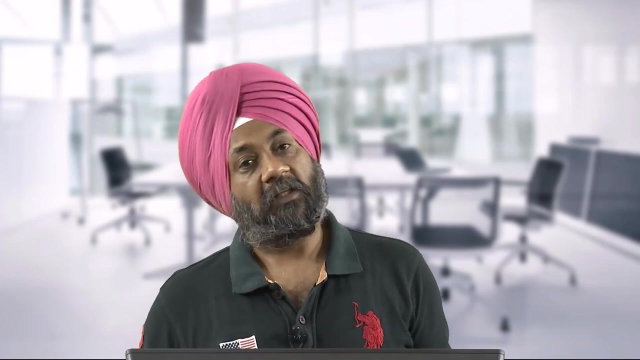 Some examples are already given, For example, ferrous metals. examples are given non-ferrous metals. examples are given Plastics. you can have different types of plastics. Plastics is itself a very large family. One classification is already given here: thermoplastics and thermosets. 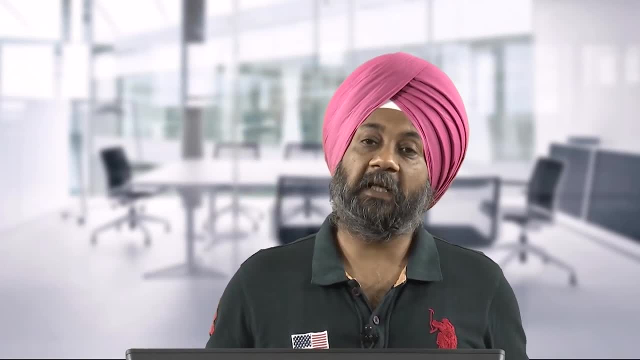 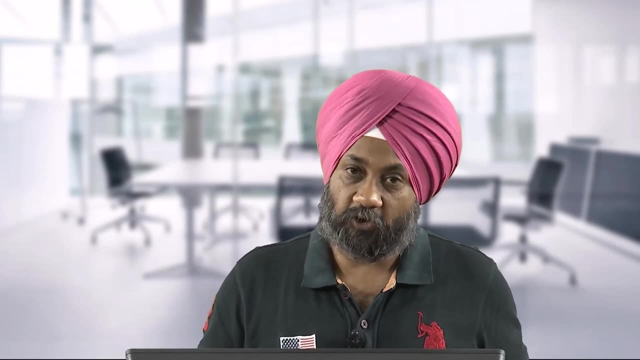 Then within thermoplastics also, you can have different types of example like polypropylene, polyethylene. For thermosets also, you can have different examples like epoxy, So you can have different types of plastics. Okay, So you can have different examples. 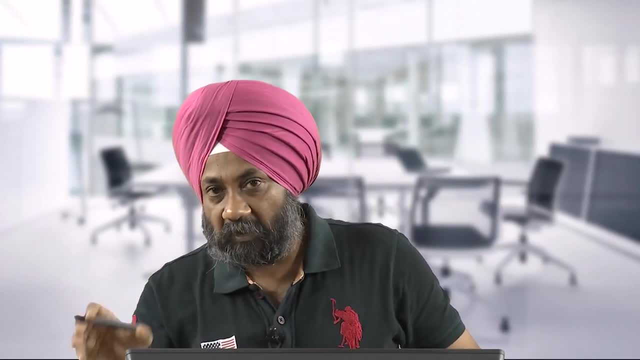 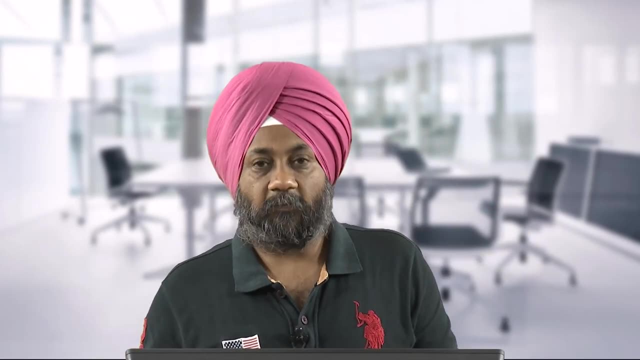 You can make a table, You can see what are the thermoplastic, what are thermosets, what are the specific application areas for thermoplastics, what are the specific application areas for the thermosets. So that kind of understanding further we can develop. 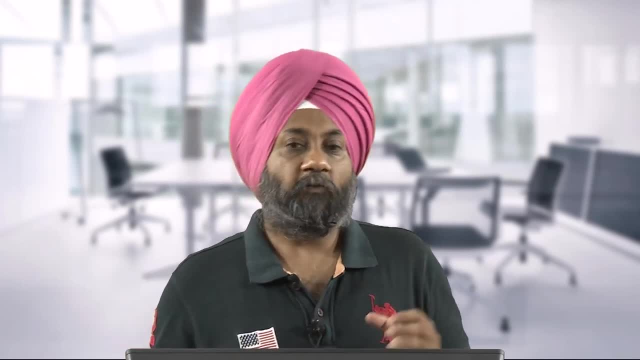 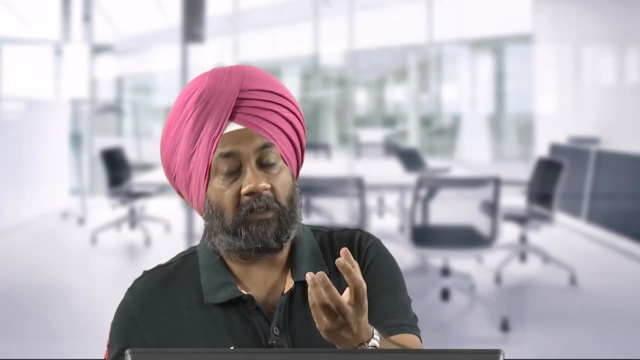 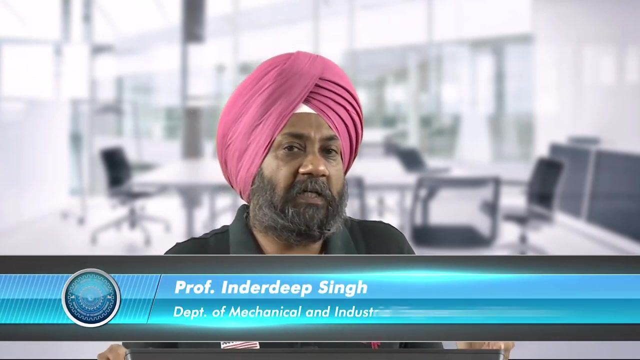 But at initial stage of product design out of this family or, sorry, out of this classification, we can choose that, yes, this particular part has to be a lot of temperature. The temperature may go up to 600 degree centigrade. So automatically, one thought must cross our mind: that polymers may not be suitable for. 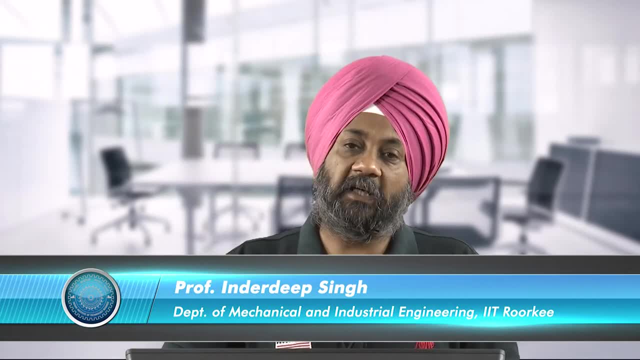 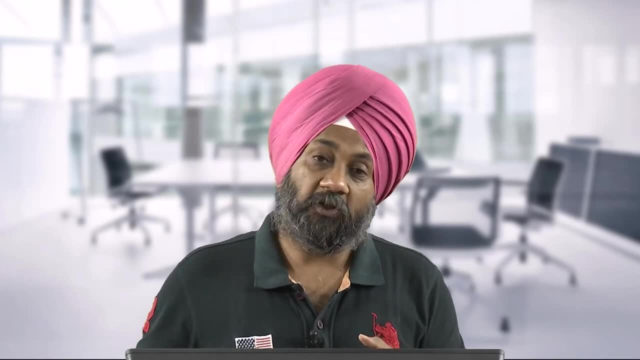 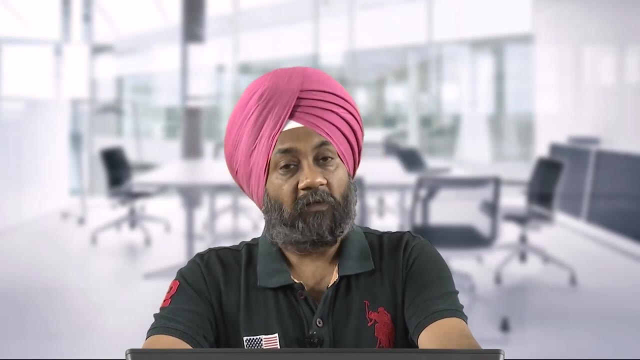 this application because it is a high temperature application. So let us propose the use of a metal for this application. and in some particular application or a product, the weight of the product may be very, very important. So we will see that polymers are best suited. 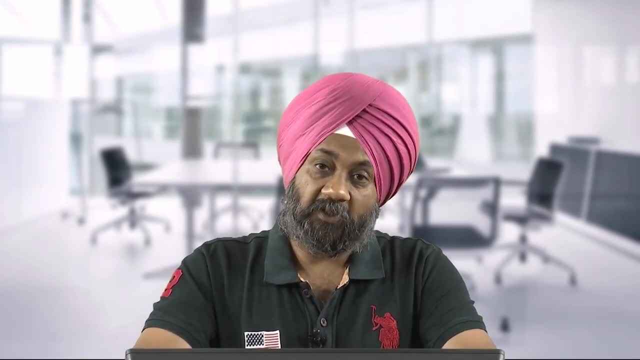 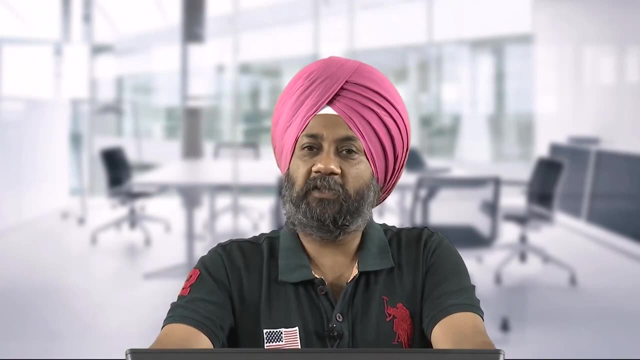 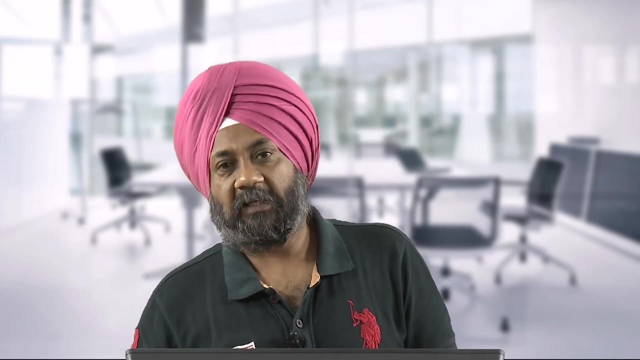 But then we will again refer to weight, Okay, Whether that temperature is going to affect any role or is going to affect and the performance of this product. We see that no, temperature is not an important parameter for this product, So then we will propose that, okay, light weight is the main criteria. 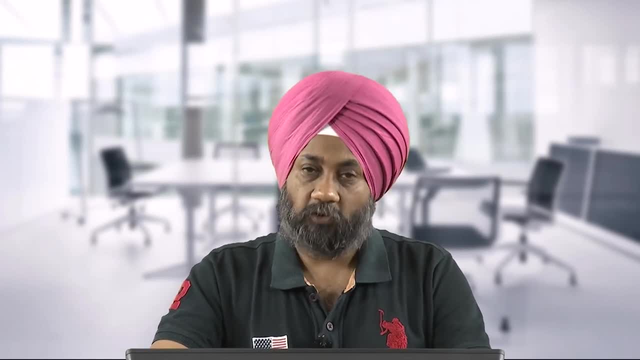 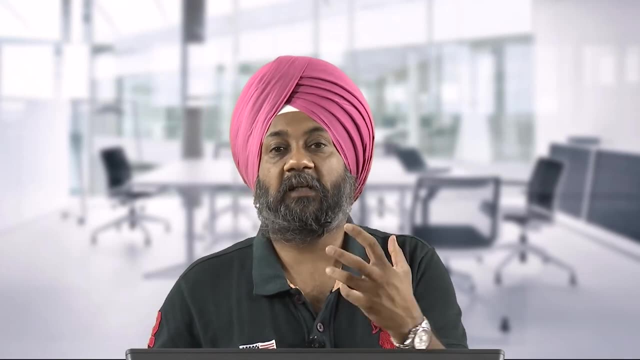 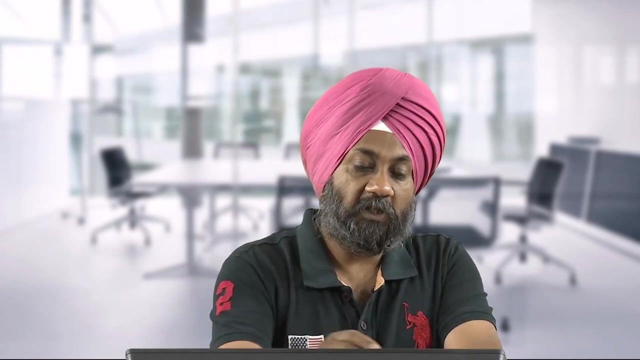 Let us go for the plastics for making this product. So that way we have to do analysis. maybe we have to give weights for the various parameters and then find out that which is the best applicable material for this Particular product. So this classification is important and each and every product designer must know that. 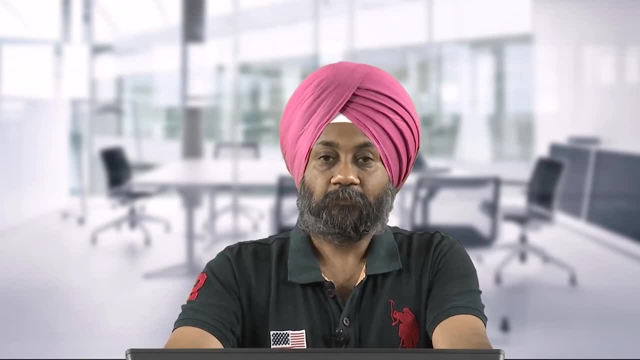 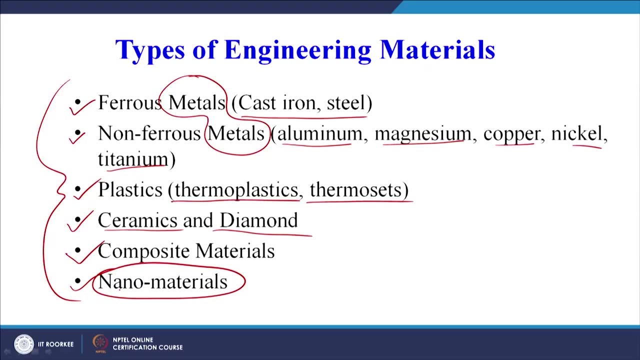 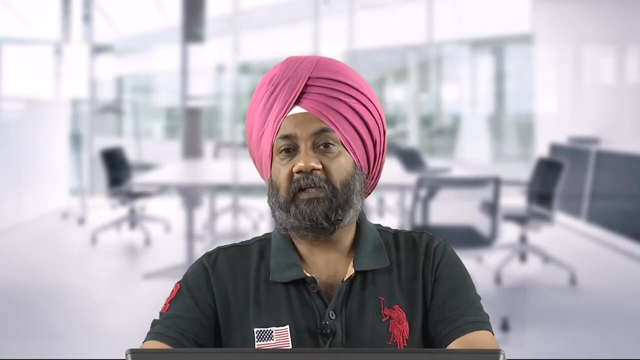 what are the various choices or what are the various parameters that are going to help him to design the product, or what are the various, we can say important class of materials out of which he or she can choose in order to fabricate the product. Now we will take each one of these very quickly. 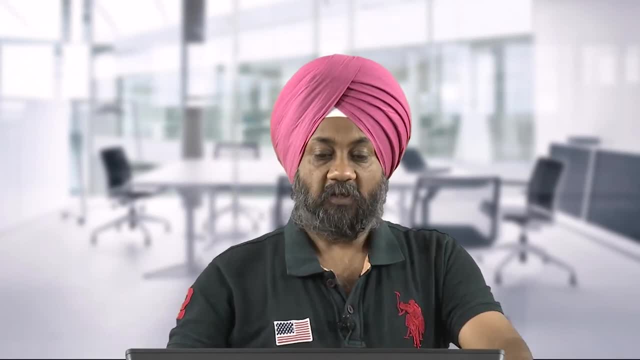 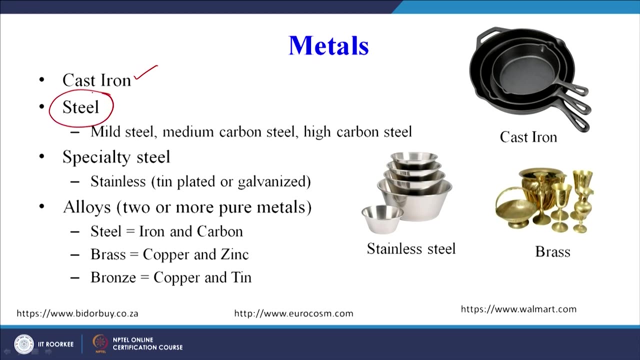 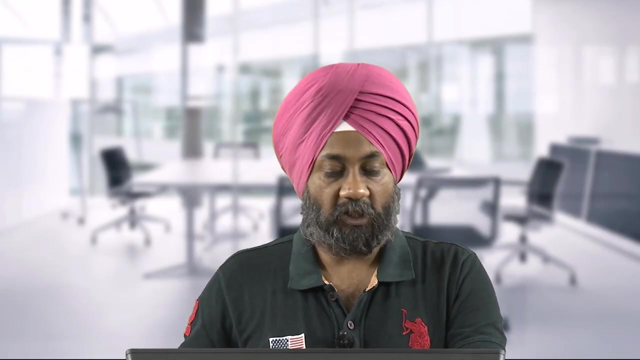 Okay, Okay With example. so metals we can see we can have cast iron, very commonly used material. all of us use steel utensils or may have used steel utensils at any given time of our lives. may be in hostels. usually we have steel plates for having our meals. 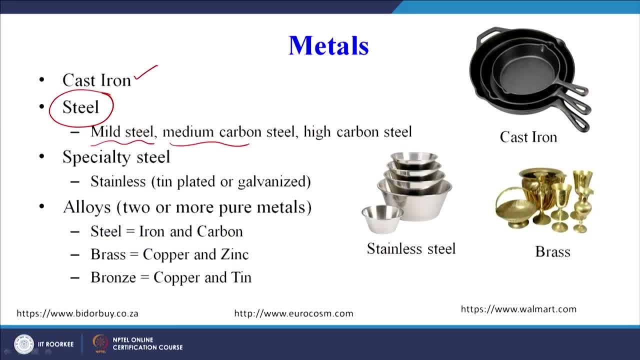 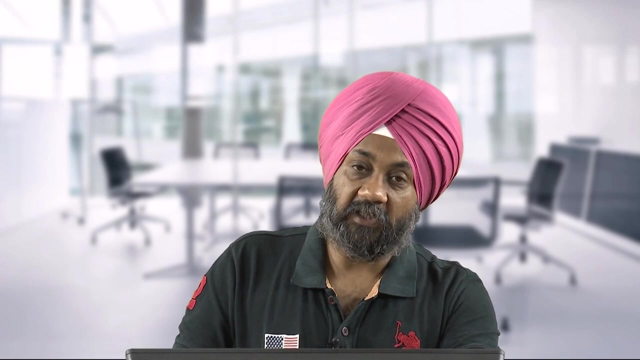 Then, within steel also, we can have mild steel, we can have medium carbon steel, we can have high carbon steel, And each one of these will have their specific application. Okay, Specific applications, so we can tailor the steel for a specific requirement. for those of you who have a mechanical engineering background, there is another type of steel which we call 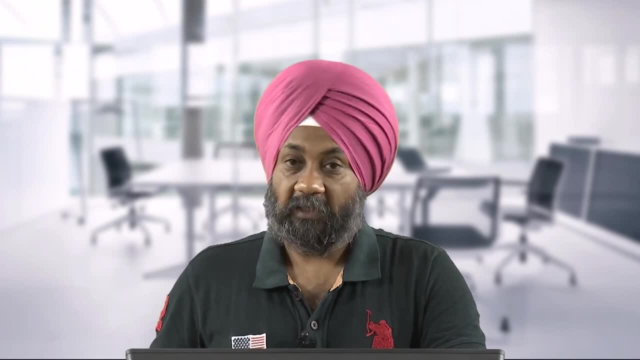 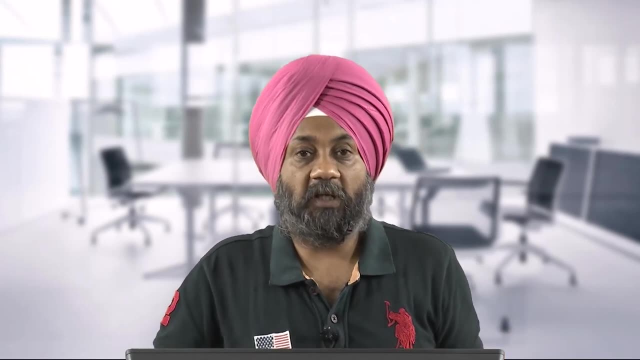 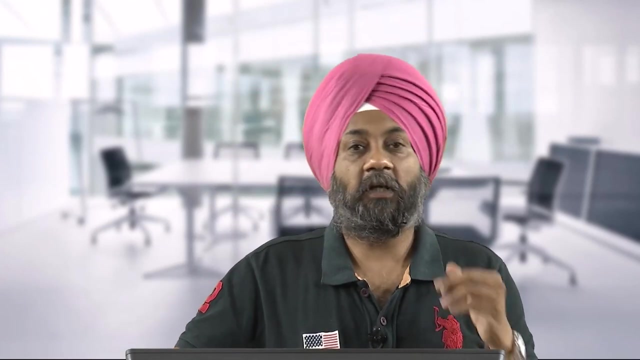 as the high speed steel which is used as a cutting tool material. So, similarly, depending upon the requirement or the application, we will see which type of steel we want to use, or which type of- we can say combination, Okay. Okay, So we can say combination of the alloying elements we have to use for a specific application. 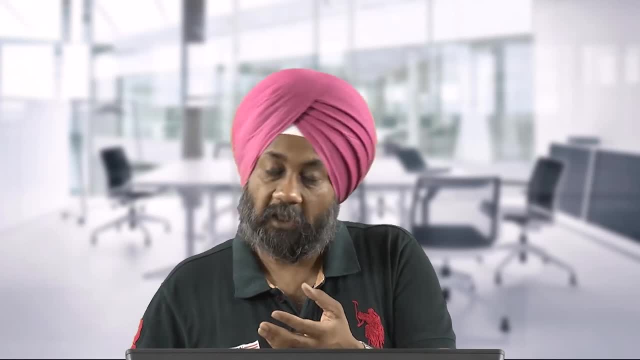 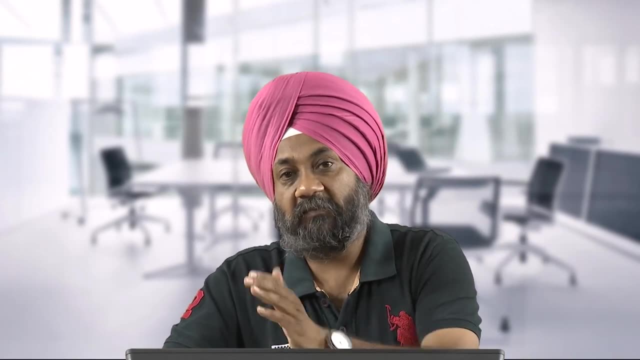 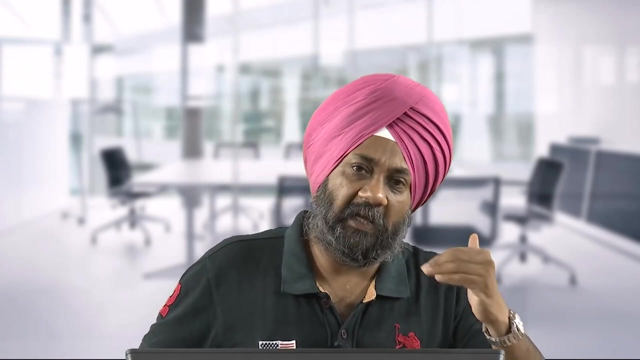 one example I have already taken as high speed steel tool. Similarly, for high speed steel also, you can further go into 1841 and see what are the various constituents or the alloying elements that make up the high speed steel. So the knowledge is endless. you can go to the any depth of understanding for any particular. 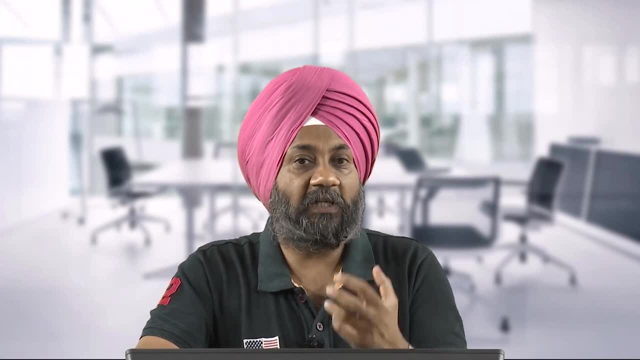 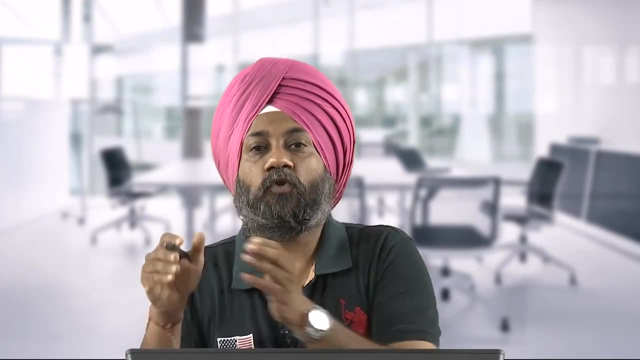 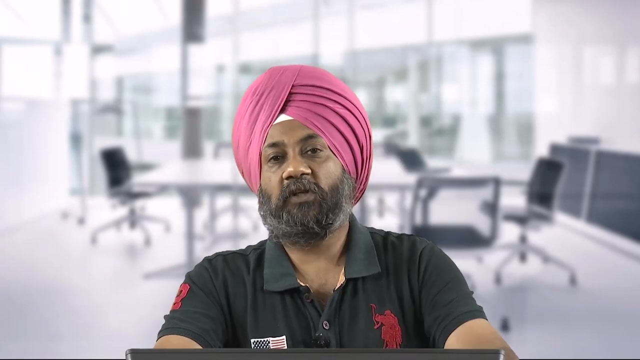 topic. So here we are just classifying now the engineering material. So if you select one particular material, for example steel within steel also, you can get handbooks on steel where a complete volume has been written on steel only and the various classification of the steels based on the different types of the alloying element. as 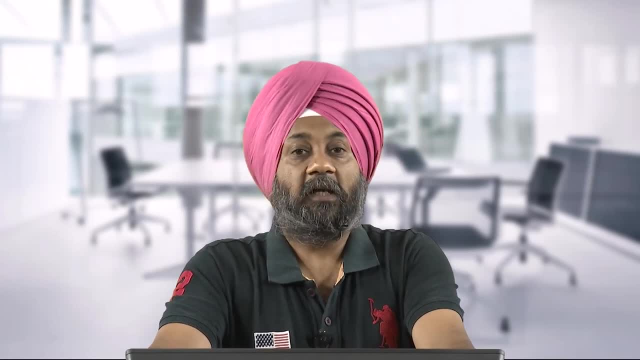 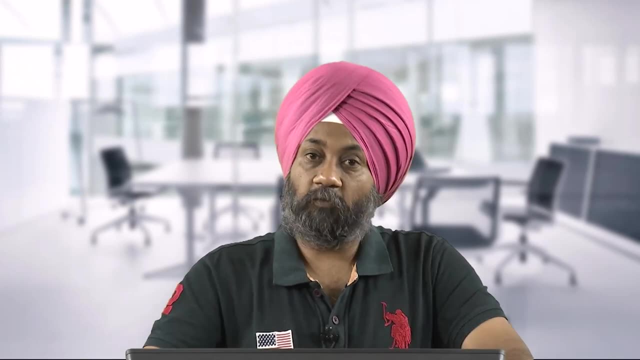 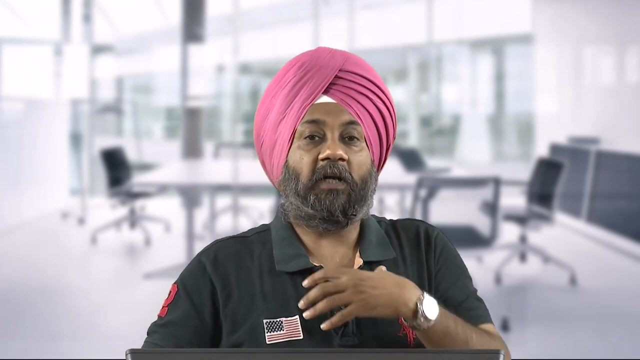 well as the application areas from the microstructural point of view, from the metallurgical point of view, from the application point of view, From the processing point of view. we can only spend maybe 20 hours or 40 hours of discussion only on steel. But as a product designer I may not be required to understand too much into steel because 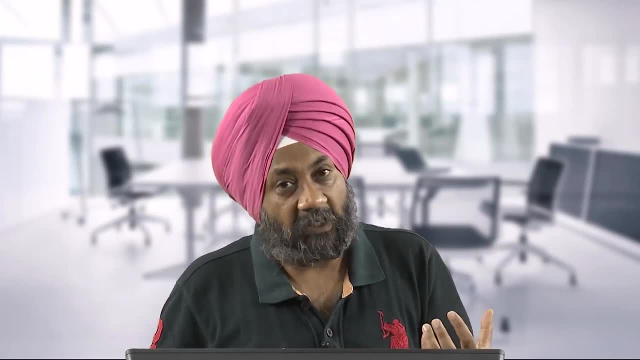 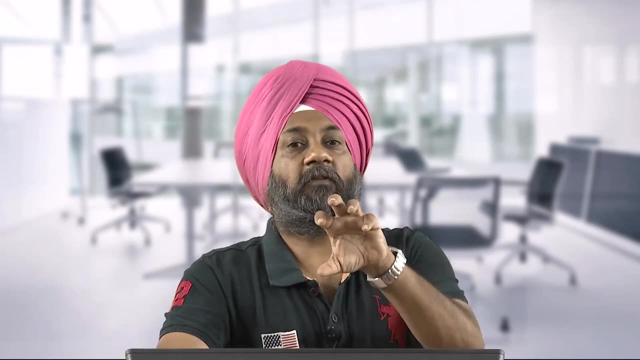 once we propose the use of steel, we can refer an expert who knows everything about steel as a engineering material and take his or her inputs when we are fabricating the product. But when I am designing, my focus has primarily to be on steel. Okay, 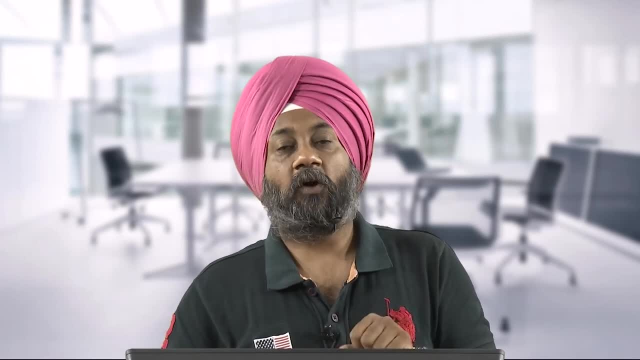 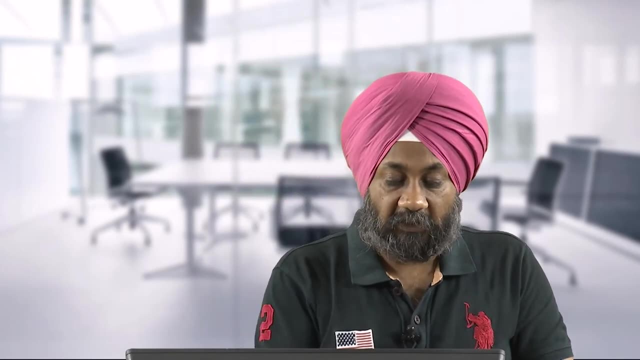 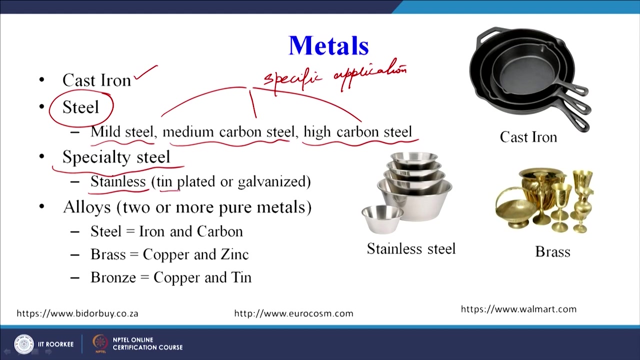 Okay, Okay, ore to be in the Vertical Aqui, Genau, Okay, Okay, it is finished. Okay, Okay. So this would be 2 útps. this is the combination of steel and ken iron. okay, or vezes, they are the same material but almost parallel to steel. 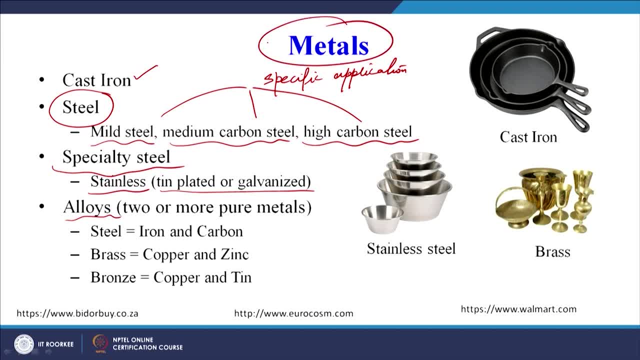 Okay, Okay. I want to Demonstrate how you can make the complete inclusive material, fights, frames, all these 2unch and mm here, So we have fully. these are the mountains here, So this is where they are. you can now we will take this as a serial material and every. 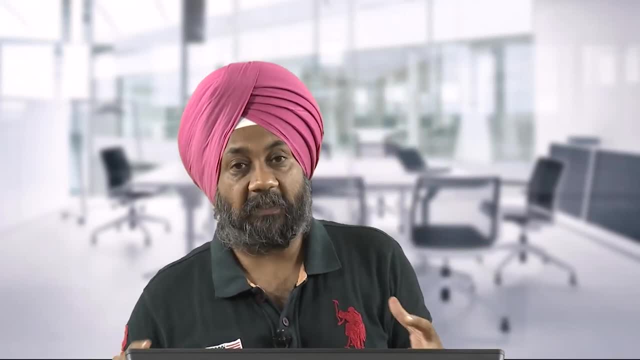 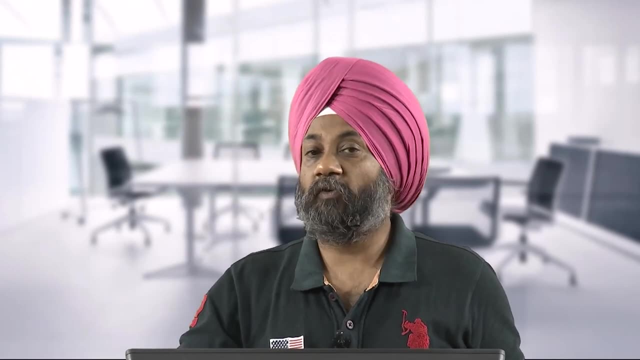 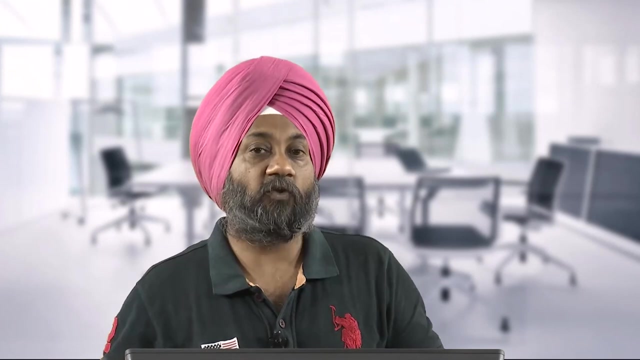 time on another plot. Okay, types of metals. you cannot use pure metals. you have to make them into alloy form for satisfying the specific engineering requirements or for specifying the manufacturing requirements. Pure metals may not be that deformable, so for making them deformable you have to alloy. 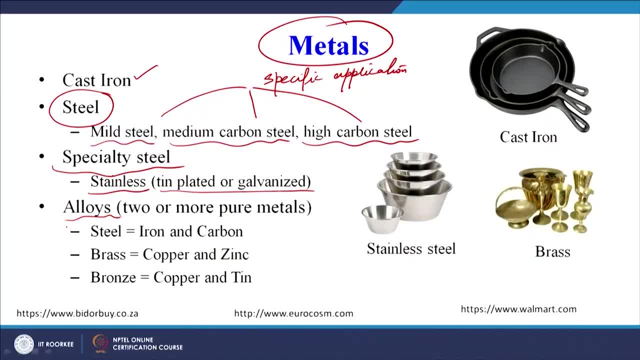 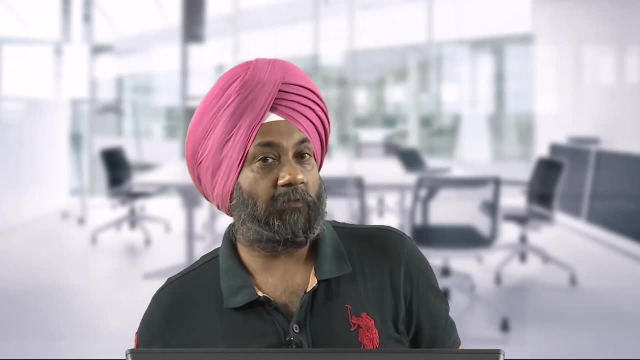 them, so you can have different types of alloys. One of the alloys example given is steel, brass, bronze, so you can have different types of alloys. So whenever we propose the use of metals within metals, also as a product designer, I may like. 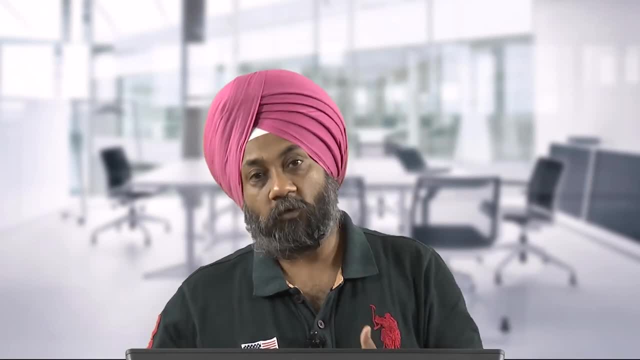 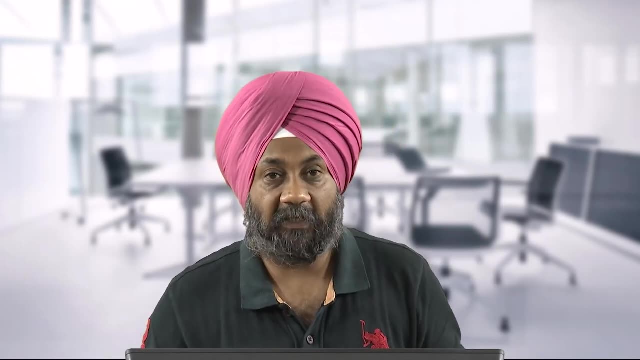 to choose from a ferrous alloy or a non-ferrous alloy. if the electricity has to be conducted, I will try to see which is the best conductor of electricity. which metal has to be chosen. If the strength is a requirement, I will see that which metal will be able to provide me. 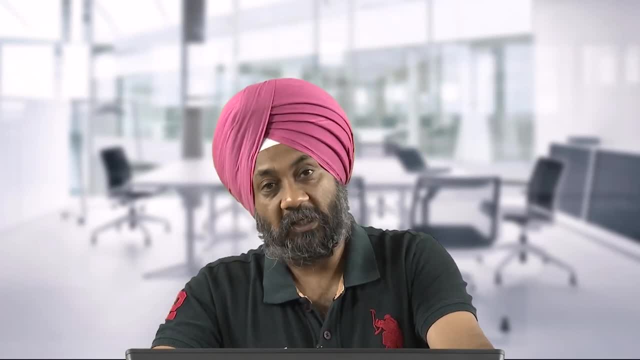 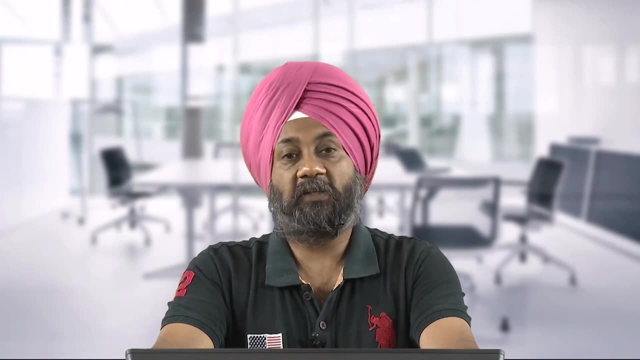 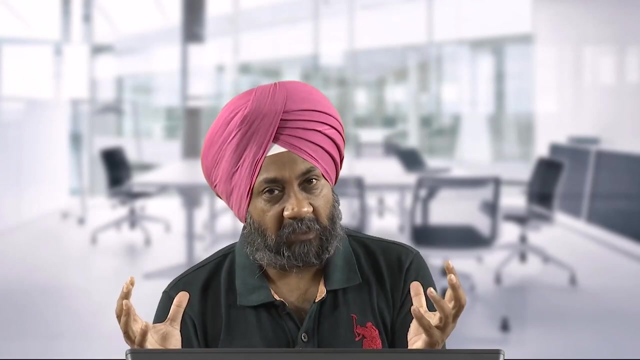 the adequate strength. if toughness is a requirement, we will see that which metal can provide us toughness. So, depending upon the requirements of the product, we can choose that which metal will satisfy our requirement. So metals is a very big family. we will try to see, if possible, during our discussion and 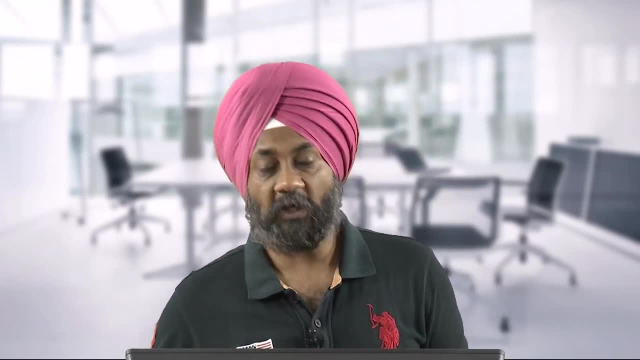 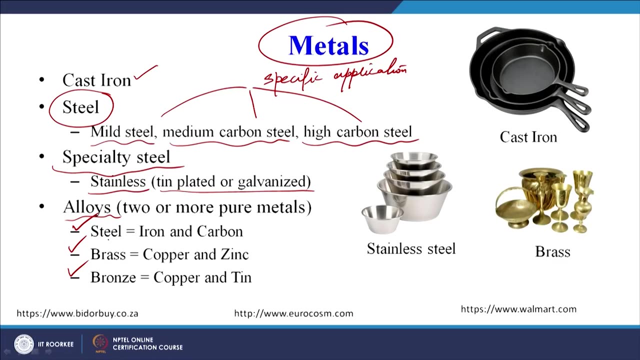 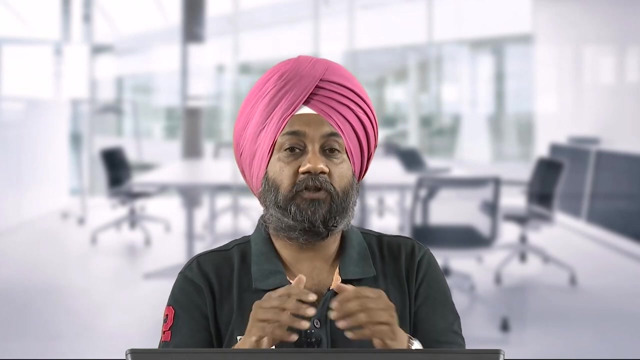 if the time permits that, what are the specific application areas for the metals- some of them definitely are mentioned here- and what are the specific properties for which the metals can be used, Or what are the specific properties for which the metals can be used, Or what are the specific requirements of the products for which the use of metals can be? 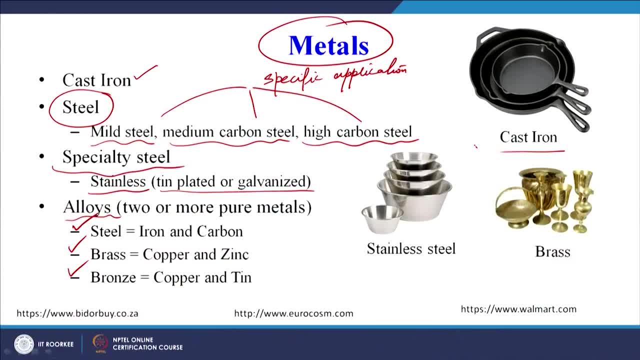 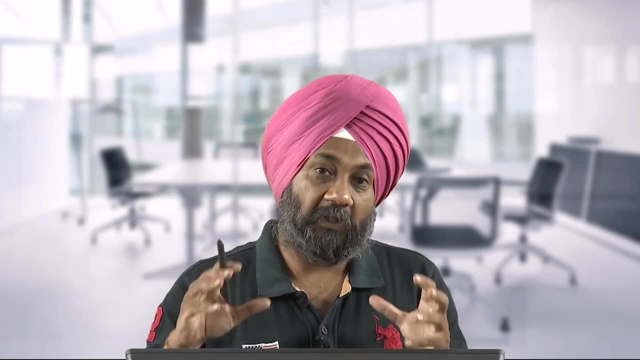 proposed. Some of them you can see here: cast iron, then stainless steel utensils, brass utensils are shown here. Then for other application different metals are used. for example the engine block is also made up of a metal, So because the temperature is higher there. so polymers cannot sustain that. so we propose: 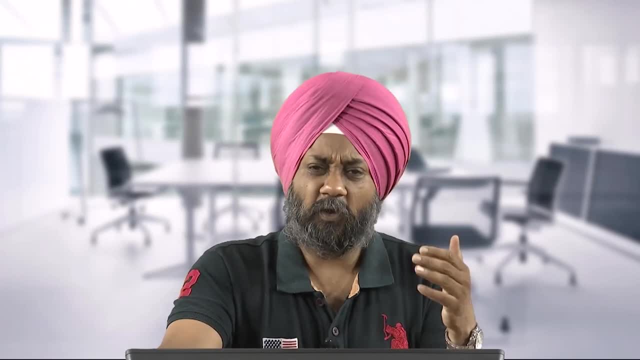 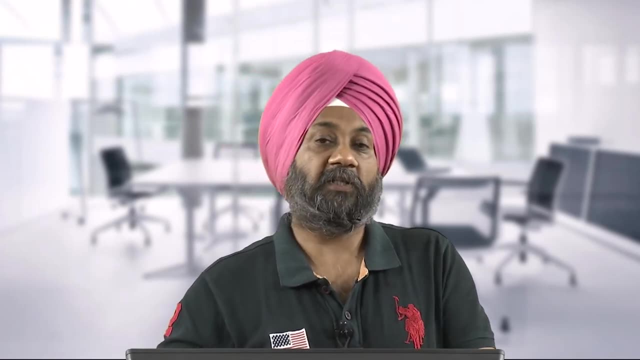 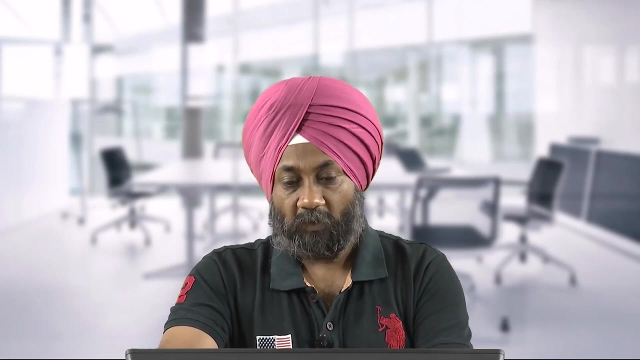 the use of a metal there. So there are number of engineering applications like connecting rod. since I am a mechanical engineer, so my examples are also related to mechanical engineering field only. So there are many applications where metals are finding use. Coming on to the polymers, there can be natural polymers like the animal cellulose then there, 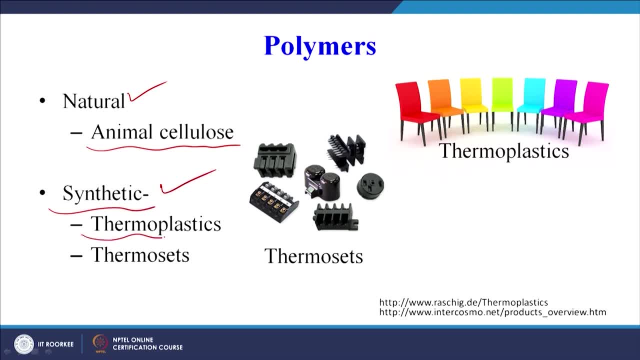 can be synthetic polymers, which we have already seen, thermoplastics and thermosets. so some of these applications are Thermoset application. these are the thermoplastic applications. Now, what is the difference between thermosets and thermoplastics? that we will cover maybe. 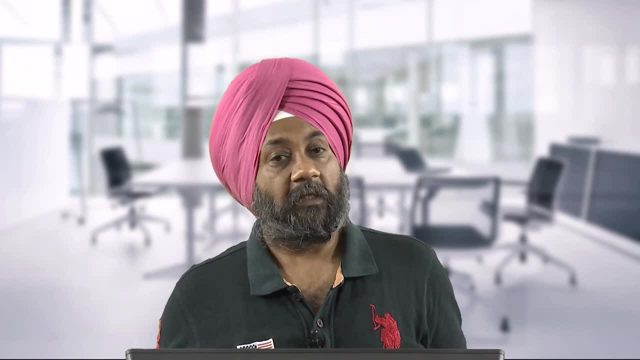 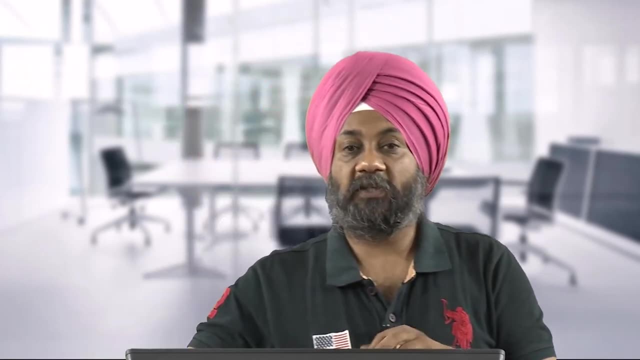 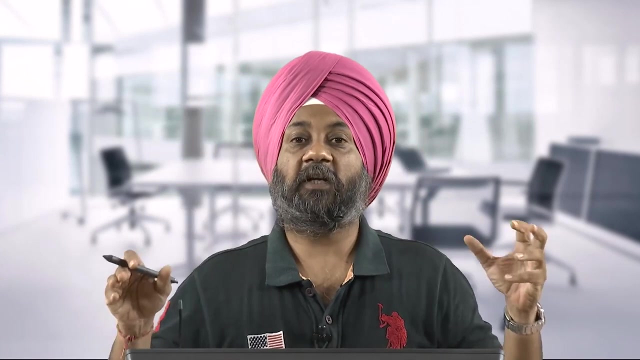 in the subsequent sessions. But polymers is a large family. it is also very, very exhaustive family. If you tell me to name maybe 5 types of thermoplastics and 5 types of thermosets, those can easily be named. why? because the family is very, very large. 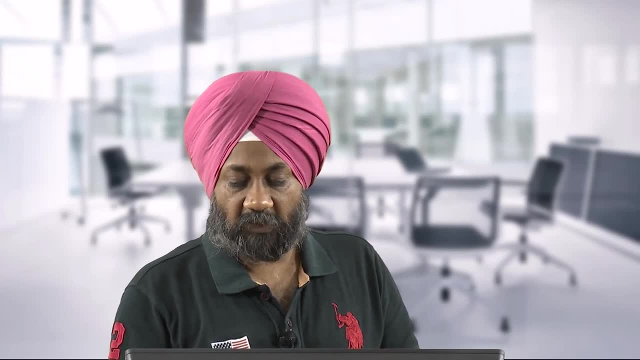 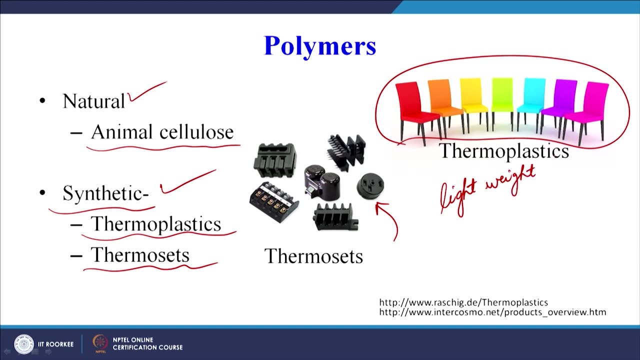 The types of polymer applications we can see. the applications are basically lightweight applications for polymers as well. as we will see that for polymers we can make them. many products can be reusable or recyclable also. So we can have the. we can propose the use of plastics. 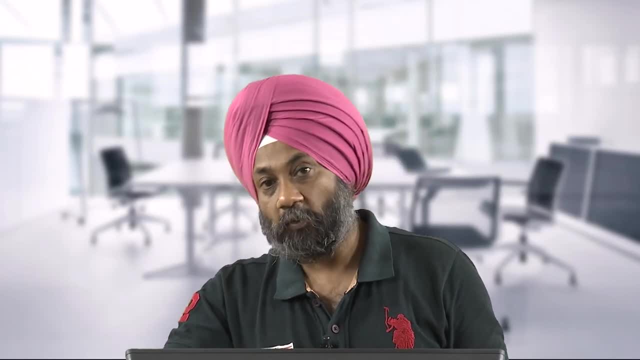 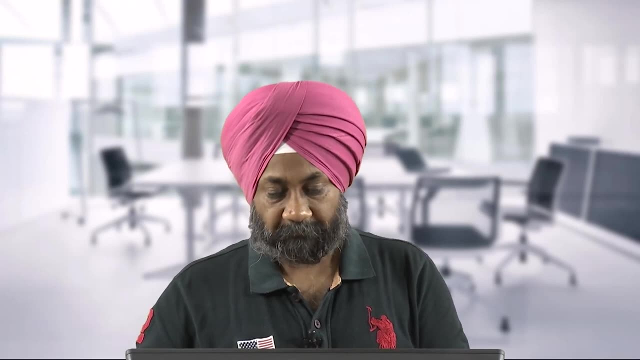 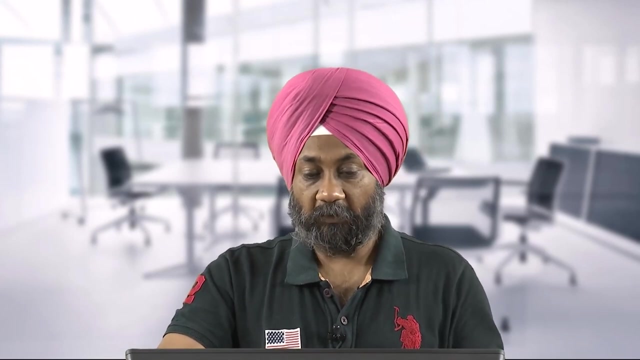 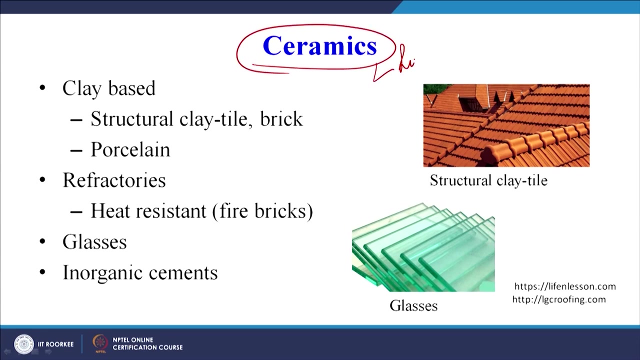 Where we want lightweight, where we want that product after its life can be recycled and a new product can be developed from the used product. so those are the application areas. We will come to the detailing in the subsequent session. Then the next category: ceramics used for basically. you will find their application for high temperatures. 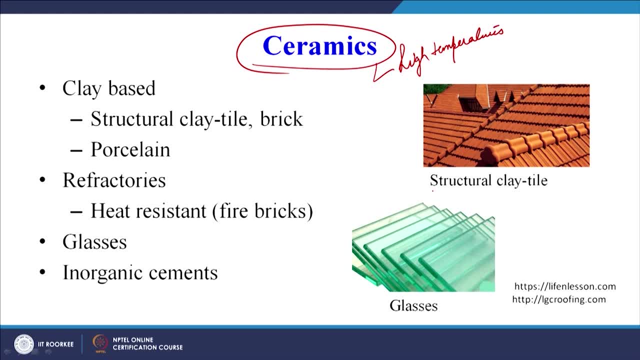 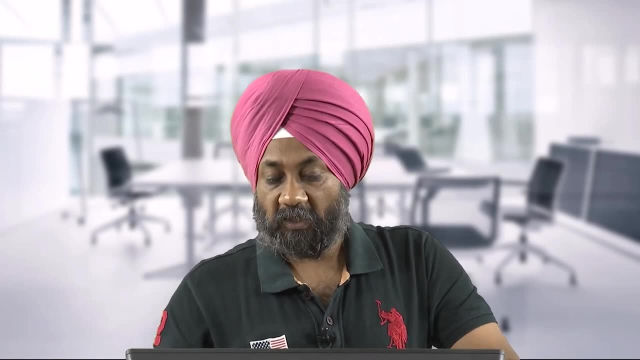 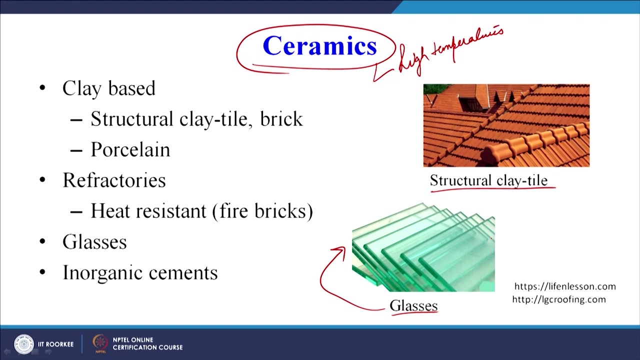 heat stress, coal, makeshift internal materials, Clothes are alltogether made by tools like glass, held in more than two columns g QUALITY OF CONSUMING G basta plus Wednesday, Christmas, june, monъ 1 en factories is another category, which have heat resistant fire bricks. glasses- another category. 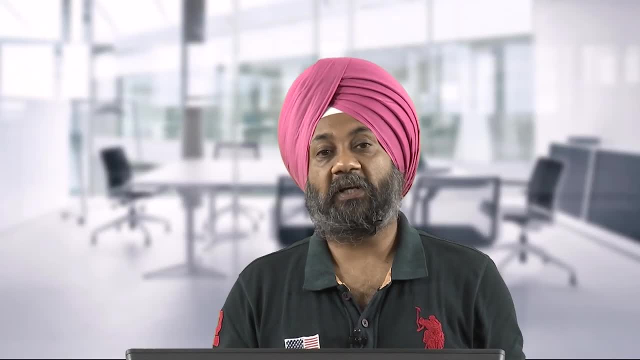 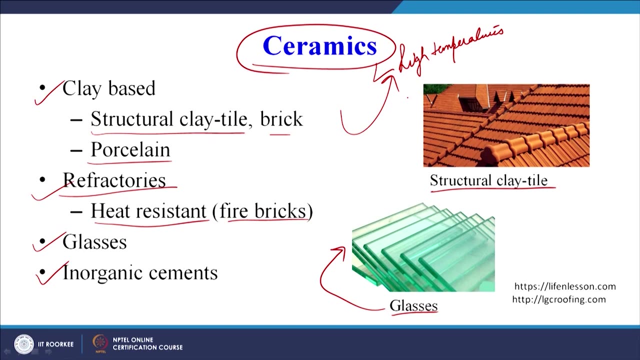 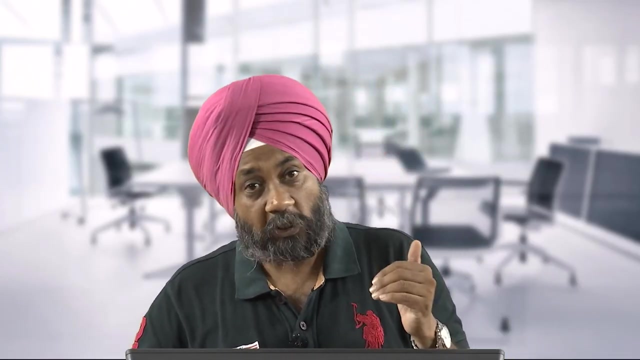 inorganic cements, So we have a large variety of applications for the ceramics also. but- one of the key words that I have already mentioned here- they are used for high temperature application. So if we are designing a product where the temperature is going to be very, very high, 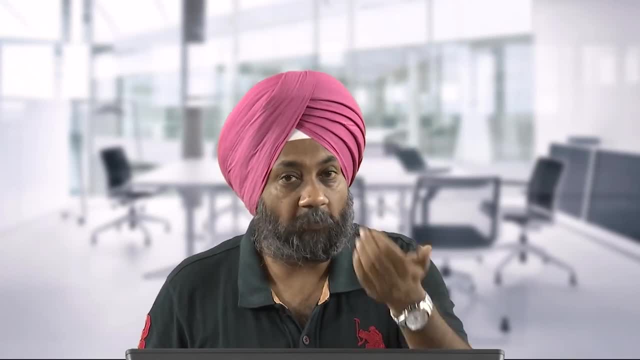 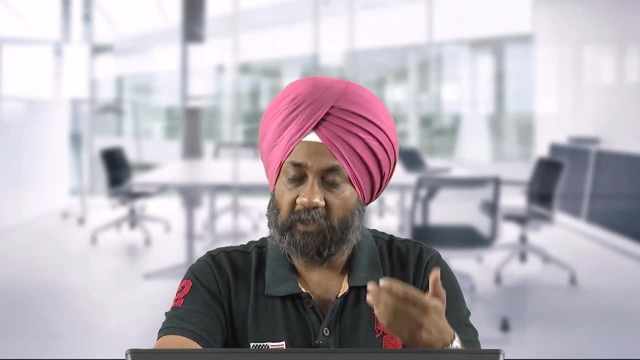 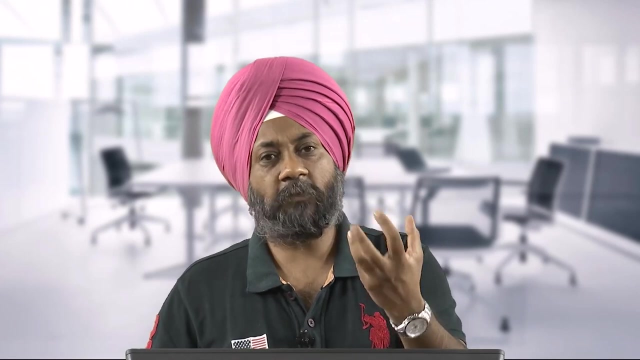 so in that case we want a material which will not deform under high temperature, and there we may propose the use of certain ceramics or certain class of ceramic material. And if one example we take, which is our day to day example, the crucibles that we use in 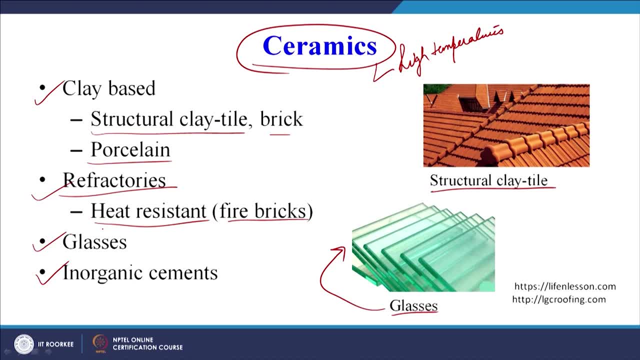 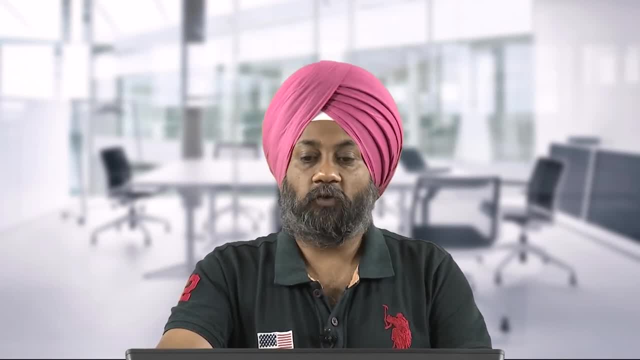 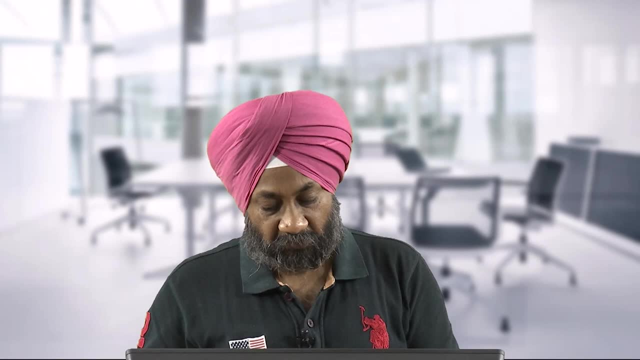 the lab experiments or sometimes some ceramic products we use in our home for serving food and other items also, which are temperature resistant. So wherever the high temperatures are used, temperature resistant materials have to be proposed. there we can propose the use of the ceramics. Then, finally, we come to another category, that is, composites. 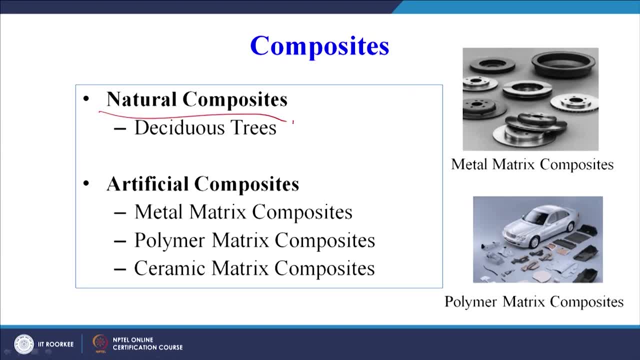 Now, composites can be natural composites. one of the natural composite, that is wood. Then there are manmade or synthetic composites. synthetic composites are of 3 types: metal matrix composites, polymer matrix composites and ceramic matrix composites. 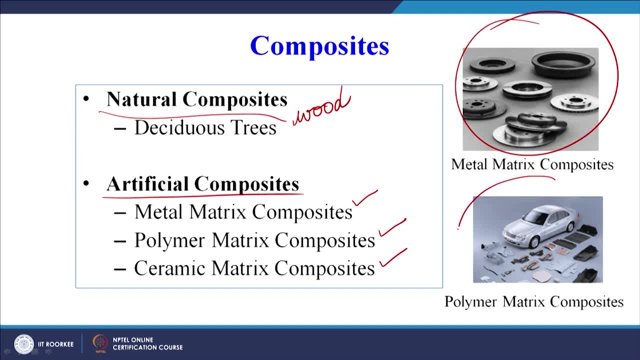 Few examples are given for metal matrix composites. These are the examples from polymer matrix composites, in which the parts that are used in making a automobile are shown here. Now, some of you may be new to this topic of metal matrix or polymer matrix composites. 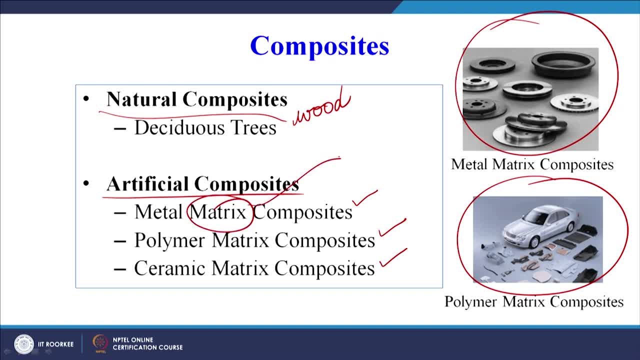 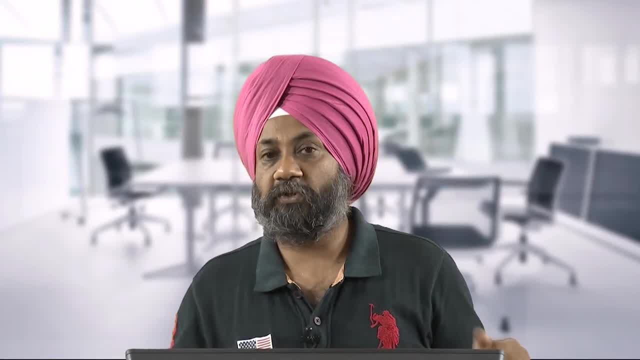 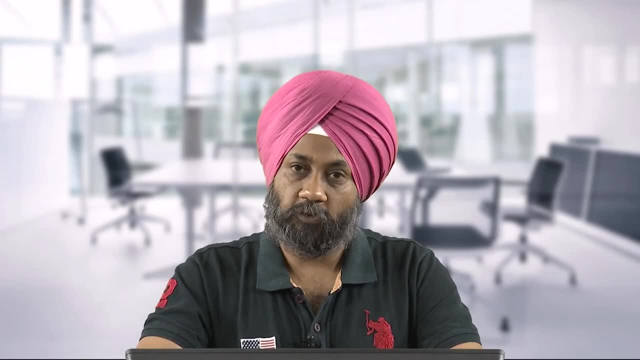 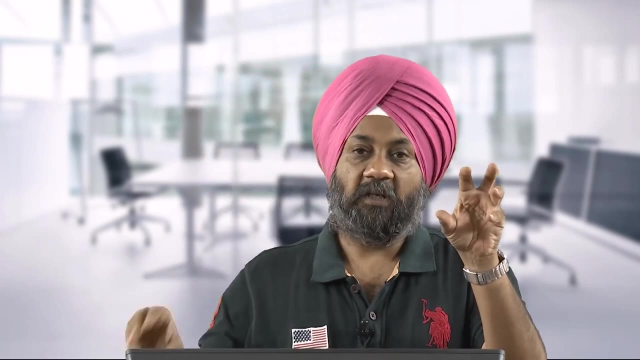 So there is an important term that is coming here, that is matrix. So if we talk of a composite material, there is a continuous phase and there is a reinforcing phase. So continuous phase is called the matrix and the reinforcing phase is called the reinforcement. So there are 2 broad, we can say- constituents in any composite material. one is a matrix. 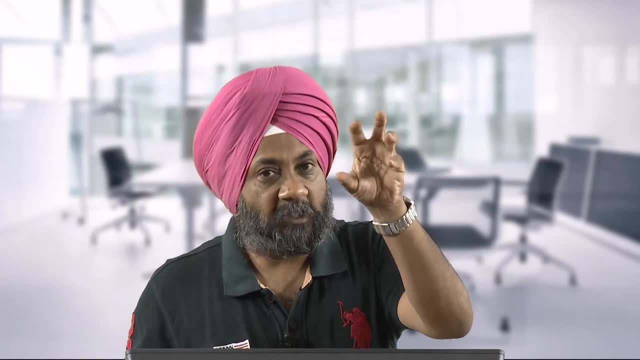 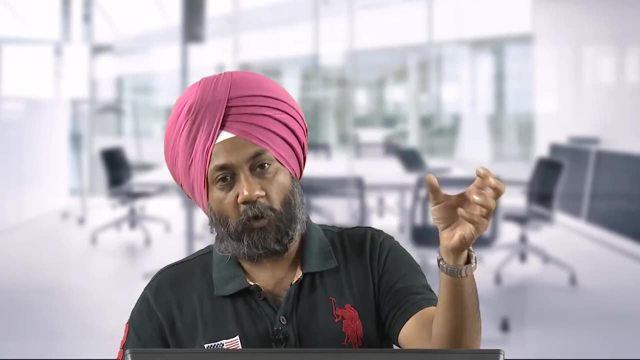 another one is a reinforcement. So from the matrix point of view, which is the continuous phase of a composite material, we can have 3 broad categories. We can have a polymer as a matrix and then we can put some fibres into this polymer and make a polymer matrix composite. 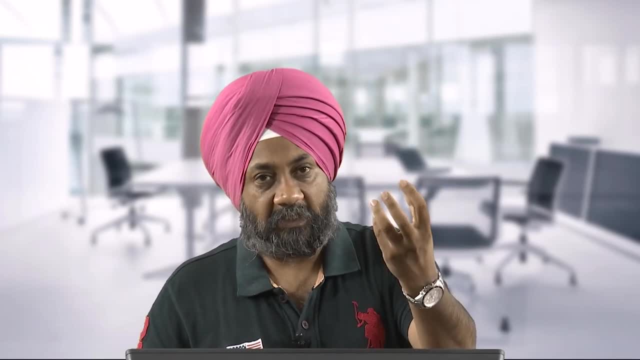 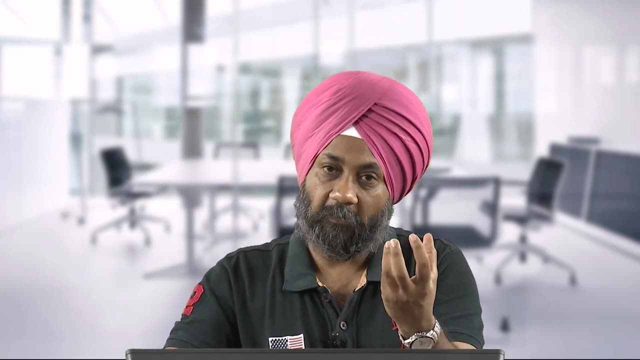 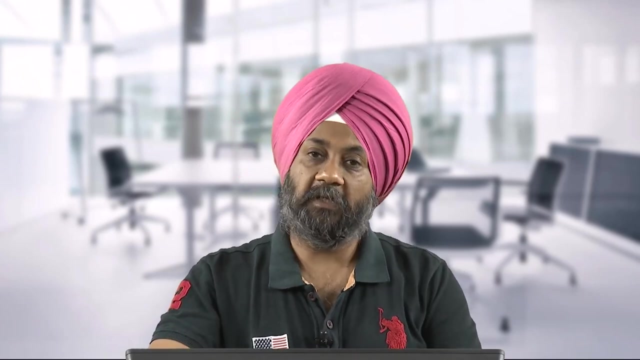 We can have a metal such as aluminum as a matrix and then we can put maybe some additive or some reinforcing agent, for example silicon carbide or aluminum oxide, into the matrix and then make it a composite material. Similarly, we can take some ceramic and then put a reinforcement into it and make a composite. 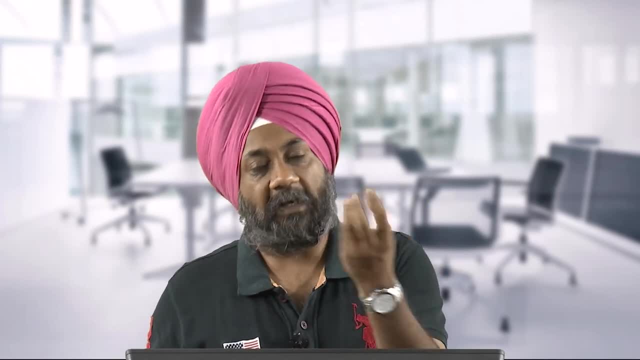 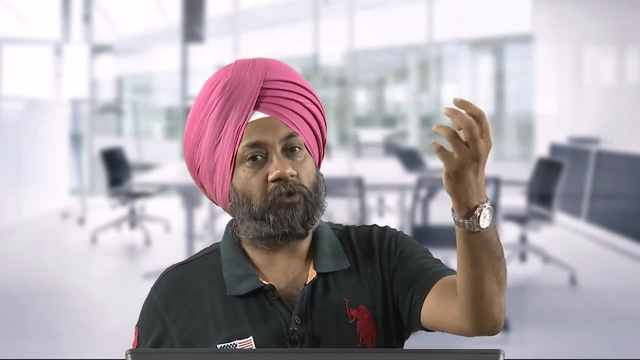 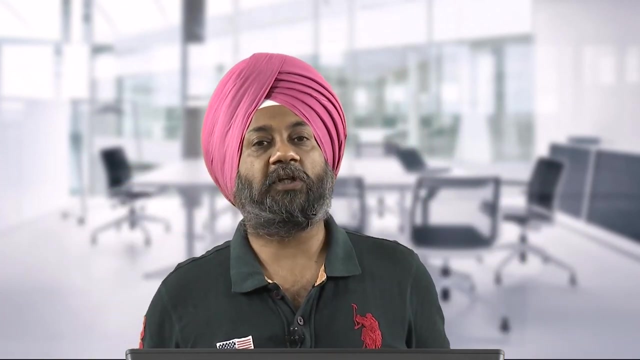 So, based on the matrix, we can have a polymer matrix, we can have a metal matrix, we can have a ceramic matrix, composite. Some of you may be wondering that when already we have a matrix, which is also engineering material, the reinforcement also is a engineering material. why do we need to combine these 2? 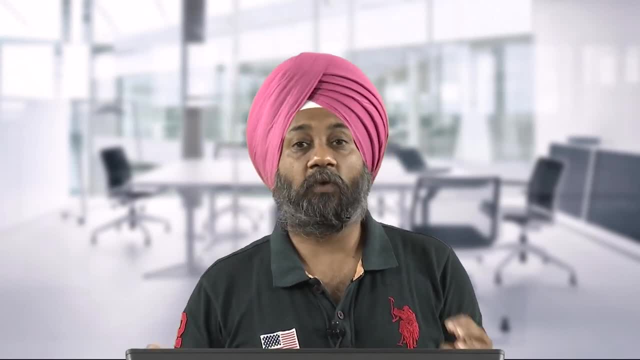 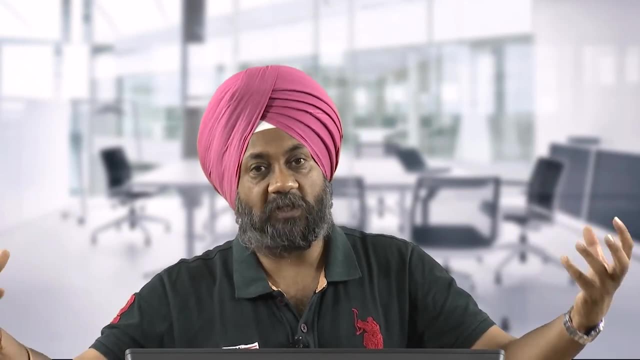 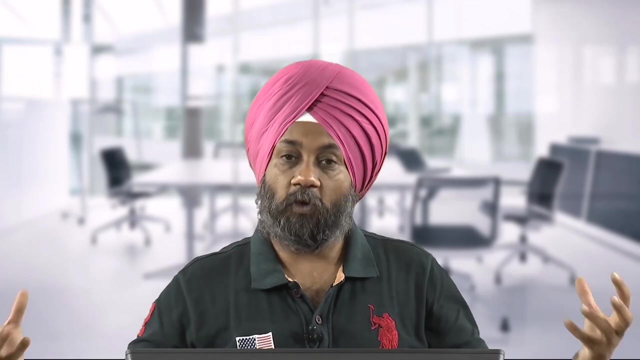 things together. Now we need to combine these 2 things together to attain the properties which are not possible with the individual constituents. So these 2 constituents may not be able to provide me the desired properties for a specific application And therefore We need to combine the 2 constituents together to make a third material which will be able 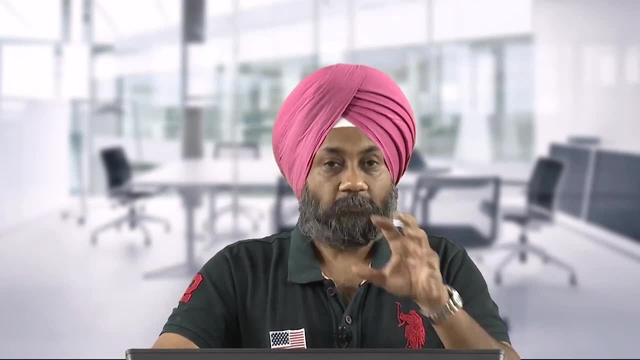 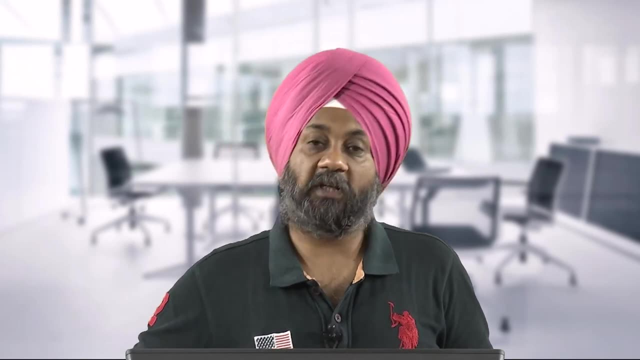 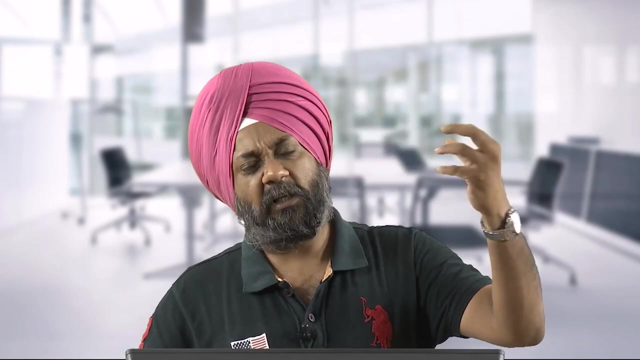 to satisfy our requirements. So that is the basic need and necessity and requirement for developing the composite materials. For example, we can say that if we want to improve the fracture toughness of a ceramic then we can add certain reinforcing agents in the ceramic. and certainly it has been proved. 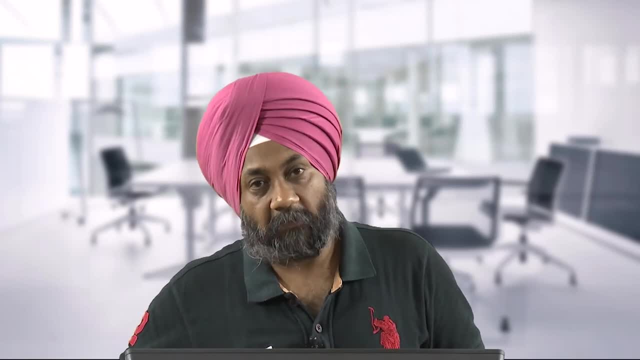 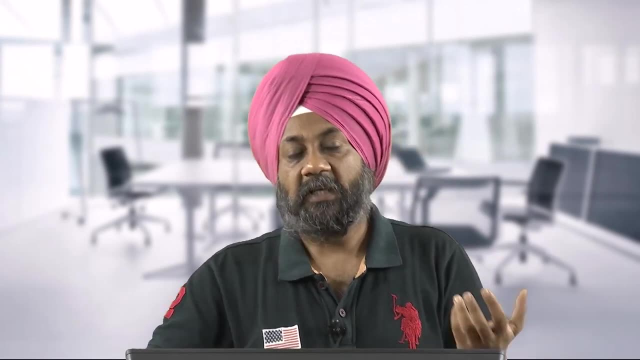 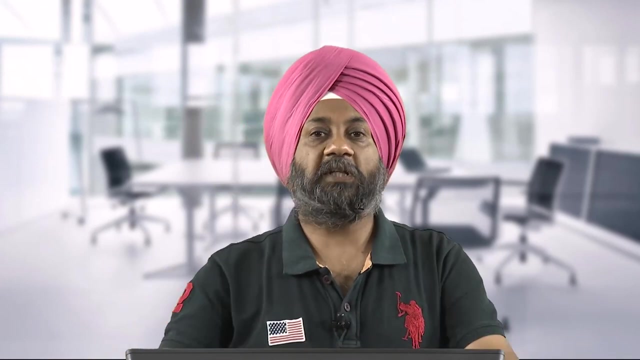 that they improve the fracture toughness, Fracture toughness of the ceramic material. Similarly for polymer also to improve its strength, to improve its tensile and compressive strength. if we add the fibrous reinforcement into the polymer, The polymer matrix composite gives us better properties as compared to the neat polymeric. 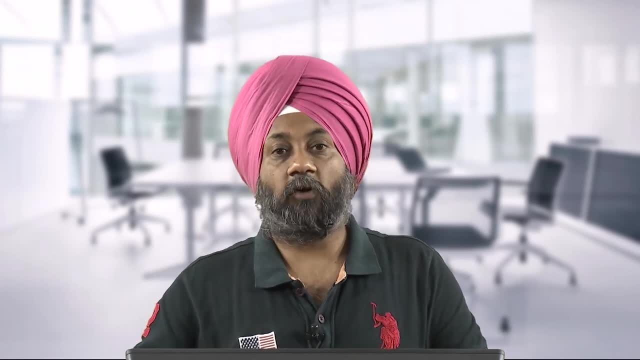 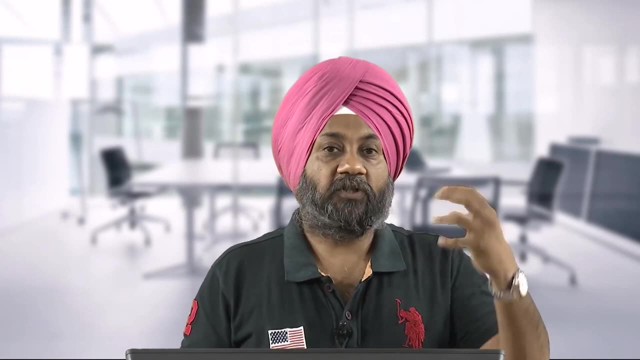 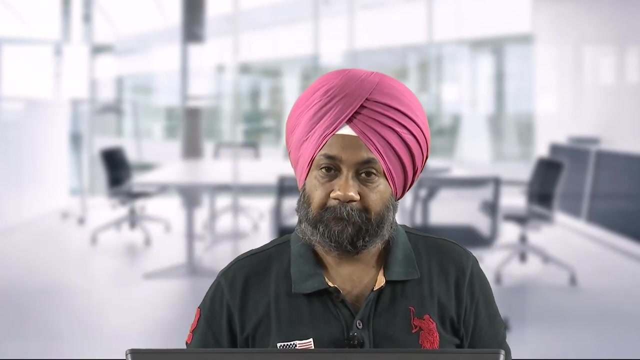 product. So therefore, there are advantages of combining the 2 constituents together and as a product designer, I must know that. yes, Instead of using a neat polymer, if I propose the use of a polymer matrix, composite, the strength, the other requirements can be extended or we can have a better product if we choose. 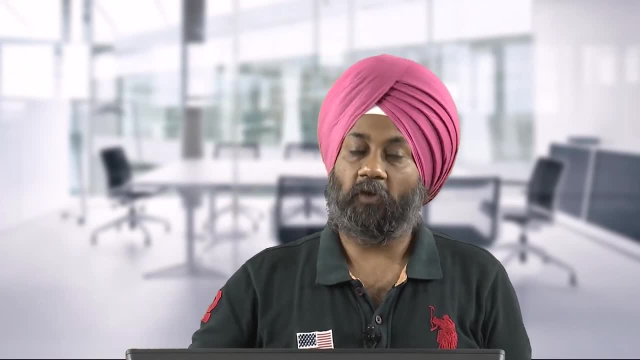 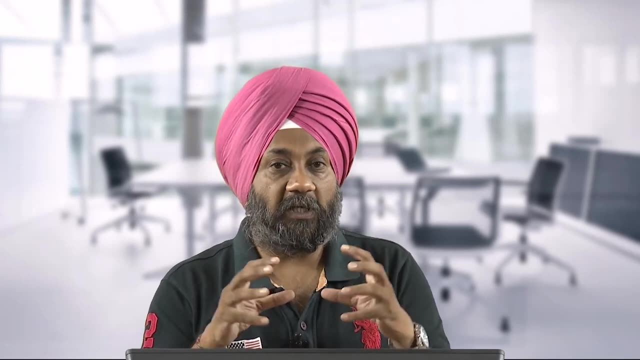 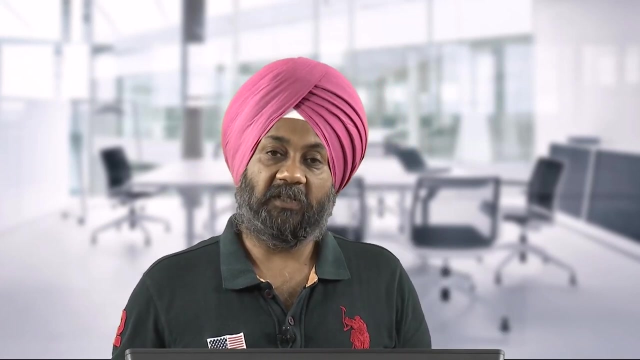 a polymer composites, as compared to a polymer or a neat polymer only. So this is another class of materials which is fast gaining applications or fast gaining importance in the engineering fraternity. So what are the challenges In selection? so the challenges in selection, I will just quickly conclude here. an ever 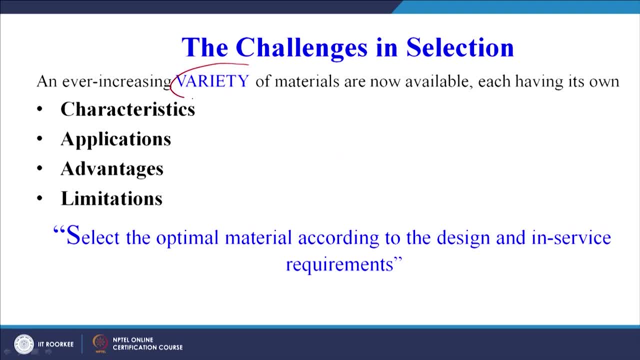 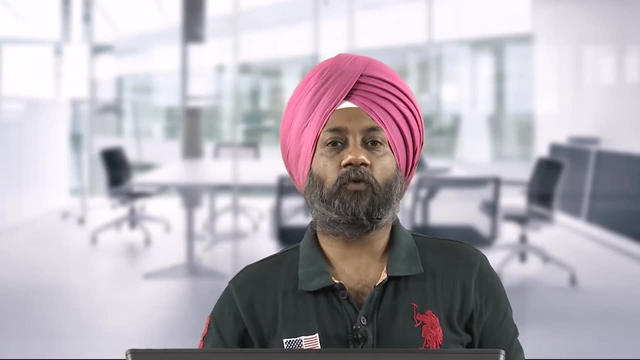 increasing variety of materials. we have seen this variety is very, very important. already in the slide we have seen 70000 types of materials are existing and the new materials are being developed every now and then. So if we have a large variety of materials, as we have seen today, also metals, which are 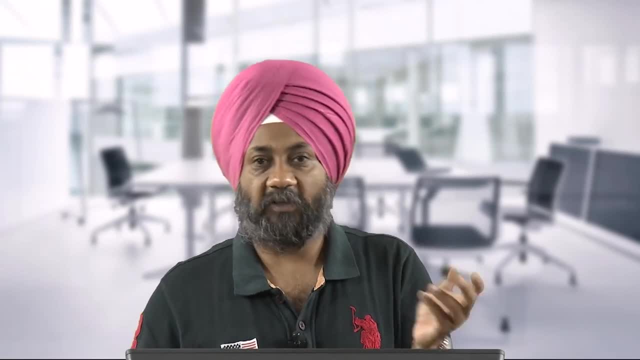 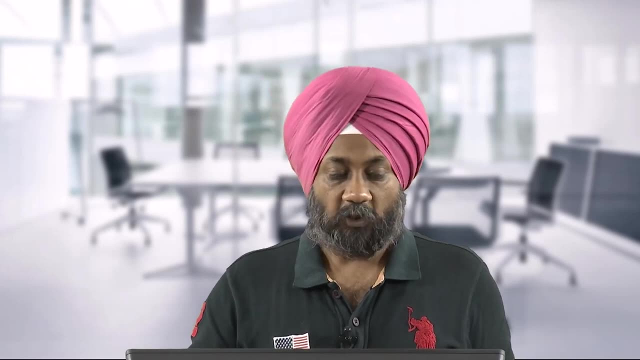 ferrous, non-ferrous, then alloys, we have polymers, we have ceramics, we have composites, We have. so how to choose that which material I must propose for my product? So for that, we need to look at the characteristics of the material, we need to look at the applications. 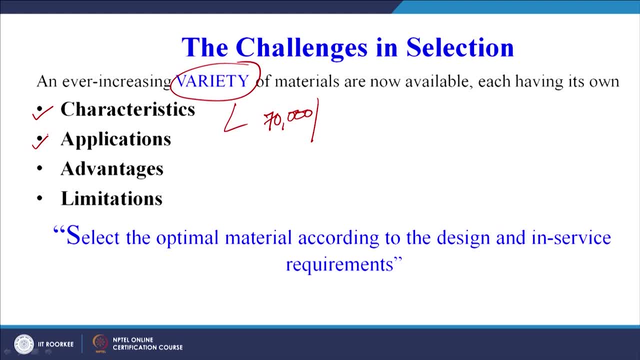 which is already prevalent in the market or which are already used for various applications or for various usages. Then we can look at the advantages of that class of materials and the limitations of that class of materials. So classes of materials already we have seen. just to have a brief summary, we can have metals. 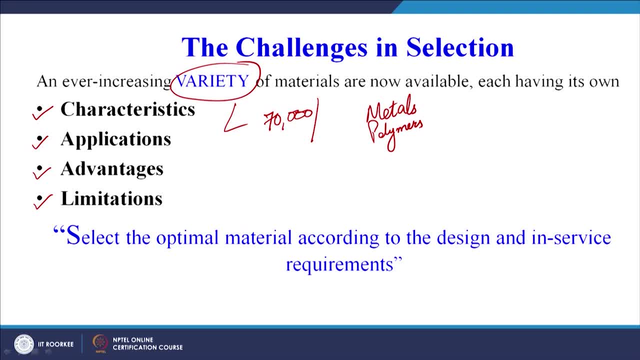 we can have polymers, we can have ceramics, we can have composites. So how to choose out of these? in order to choose, we need to look at these important parameters: the characteristics of the material, the applications, the advantages and the limitations. So, class of materials: already we have seen, just to have a brief summary, we can have metals. 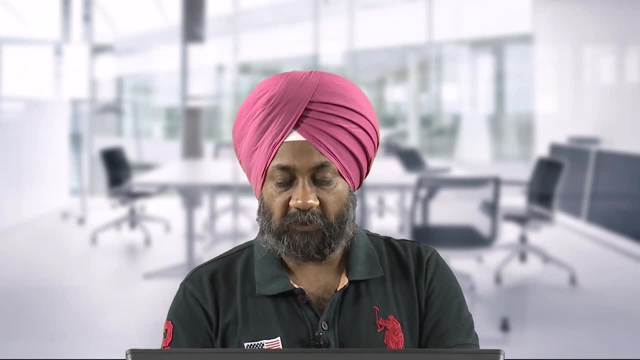 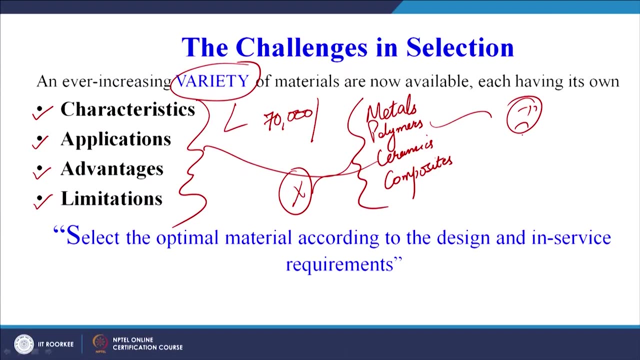 we can have polymers, we can have ceramics, we can have composites. so how to choose out of these? For example, ceramics may have got their own limitations. similarly, polymers may have their own sad points. So the polymers may not be cure for all types of applications. you cannot propose the use. 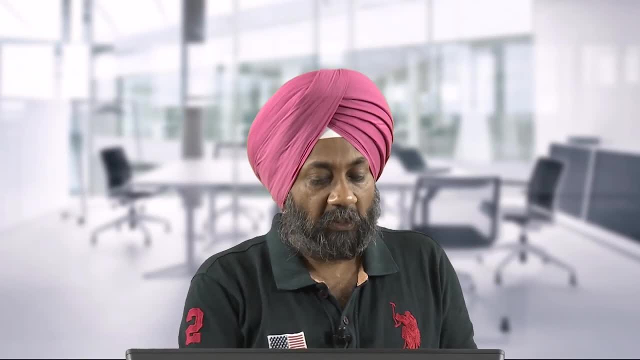 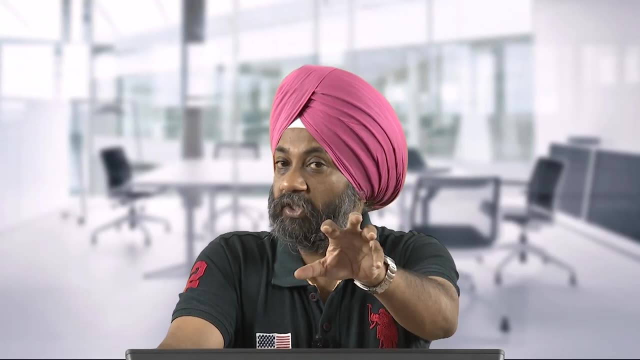 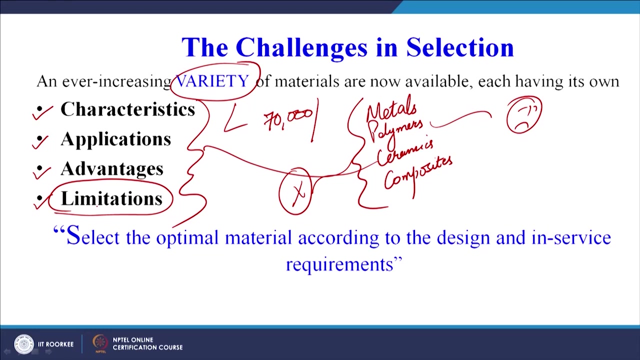 of polymers for each and every application. So we have to see their limitations also. So these limitations then become a guiding force that, yes, in this application this material cannot be used. So select the optimal material, So according to the design and in service requirements. 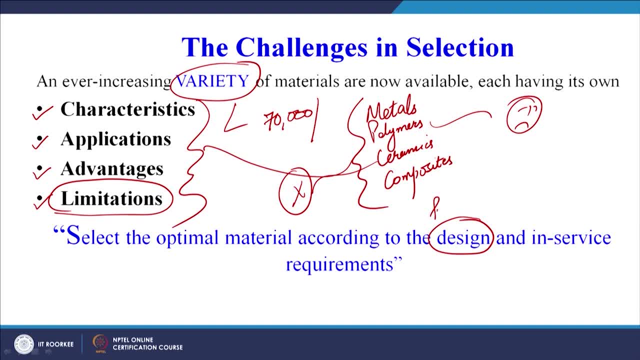 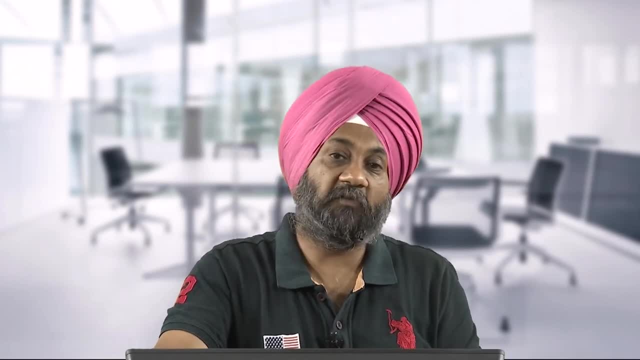 So we have to see our product design, that how my product is going to look like, what are the various features, what are the various shape requirements, what are the various size requirements. So that product design specifications we need to understand and, based on that, we need to 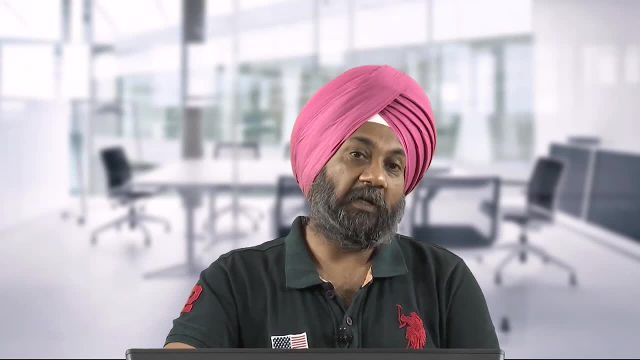 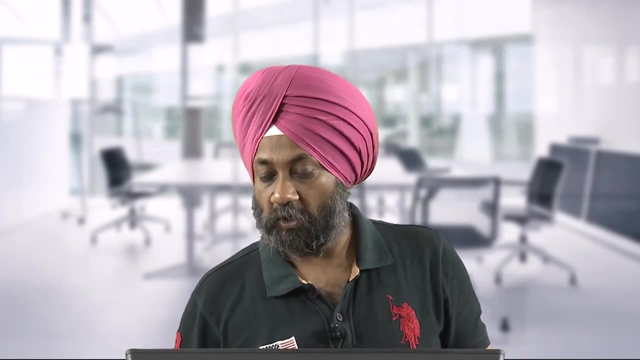 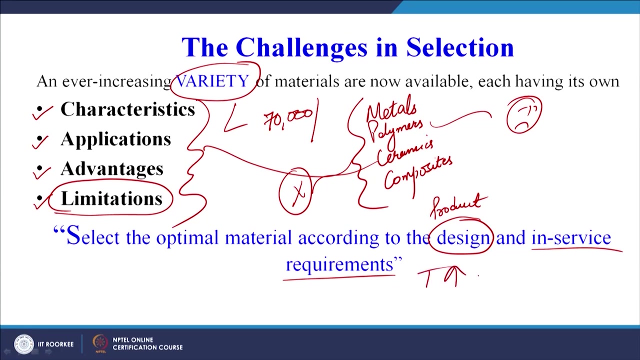 select our engineering material. also the in service requirements, As I have already Discussed when we talk of ceramics, they are good for high temperature applications. So if in in service requirements high temperature is going to be encountered by the product, we can propose the use of ceramics as the engineering material. 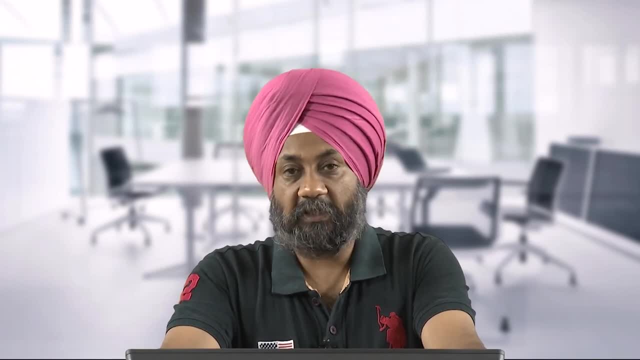 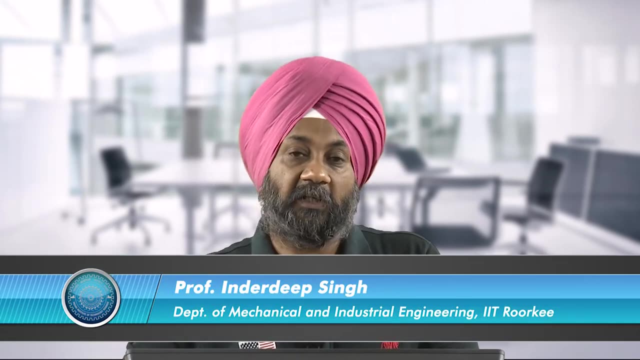 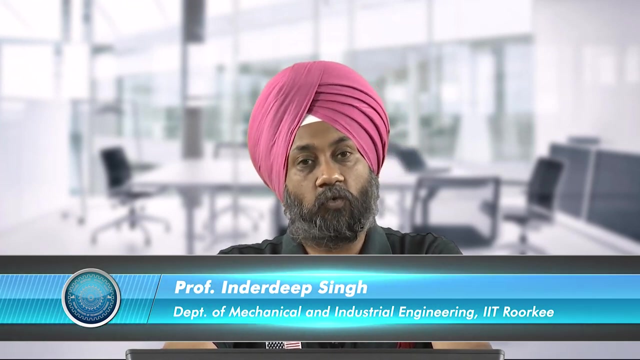 So with this we conclude the today's session, the introductory session for week 2 on engineering materials. in the next session we will carry forward our discussion related to the choice of the engineering material, That how we can decide what are the parameters governing the choice of a particular engineering. 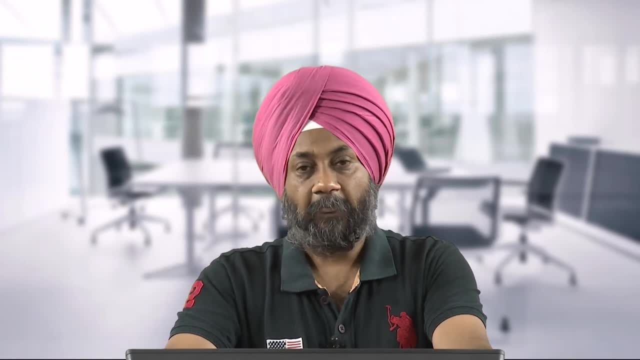 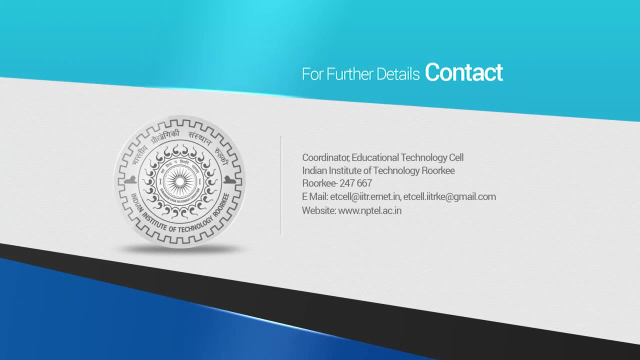 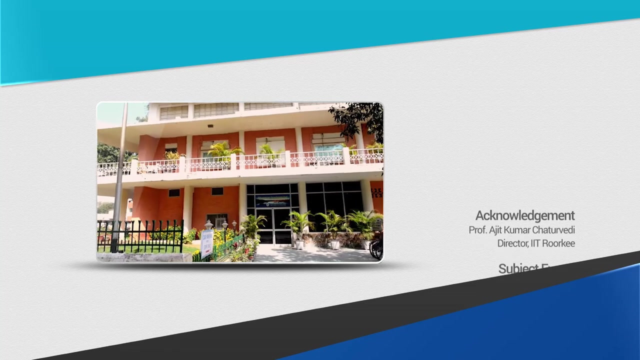 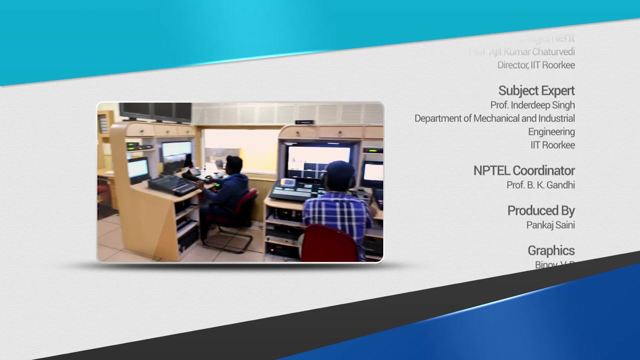 material for a particular type of product design, as well as the in service requirements. Thank you.